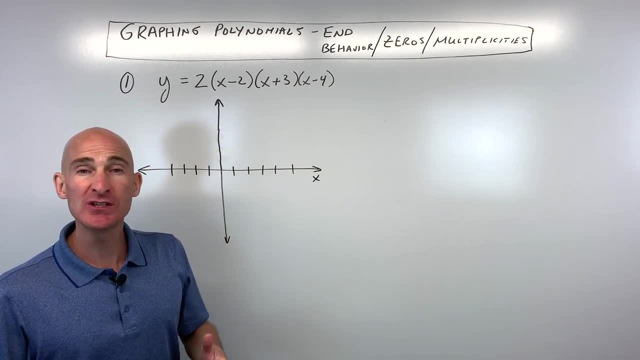 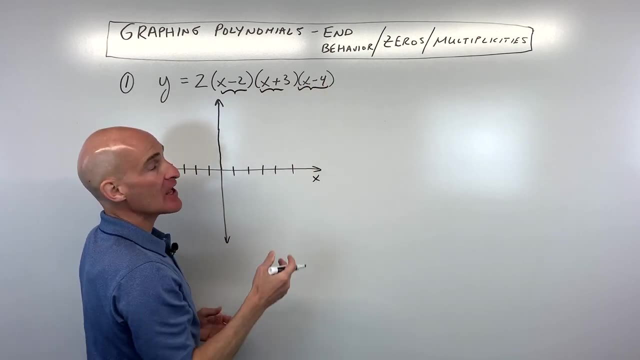 Now, this one's already in factored form, And the first thing you want to do is you want to find the zeros And to find the zeros. what you do is you take each of these groups, each of these factors, and you set them equal to zero. 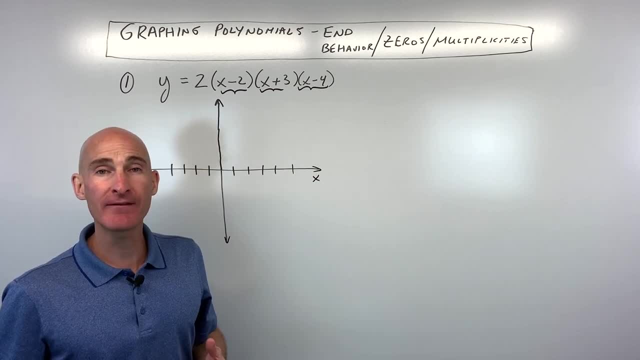 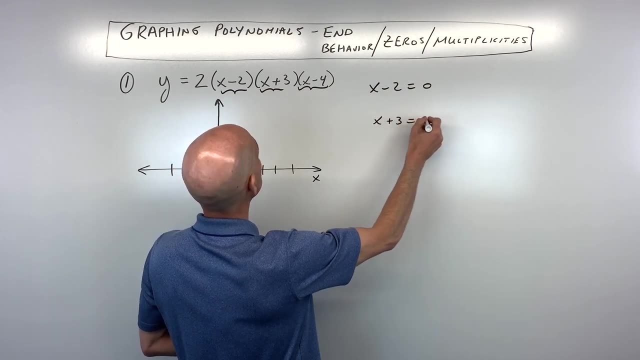 Now, if it's not factored, if you can go ahead and try and factor it, And we'll do that in the next example. So here you just make like a mini equation: x minus 2 equals 0, x plus 3 equals 0, and x minus 4 equals 0.. 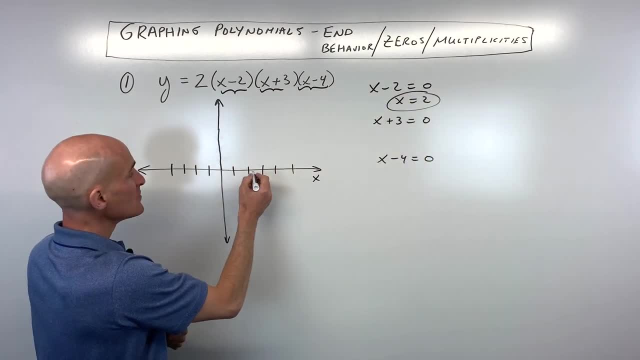 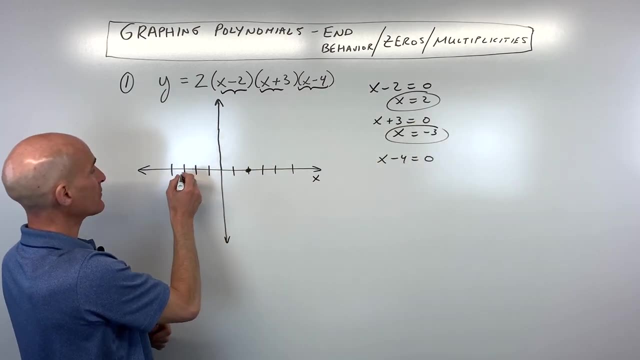 And when you solve these you can see you're getting x equals 2, which means it's going to cross the x-axis right here at 2.. Over here, when you subtract 3 from both sides, you get x equals negative 3, so it's crossing here. 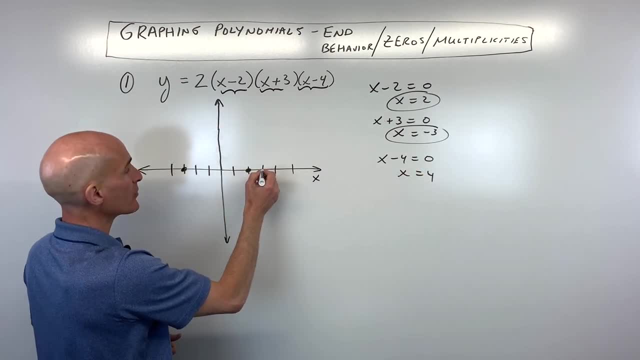 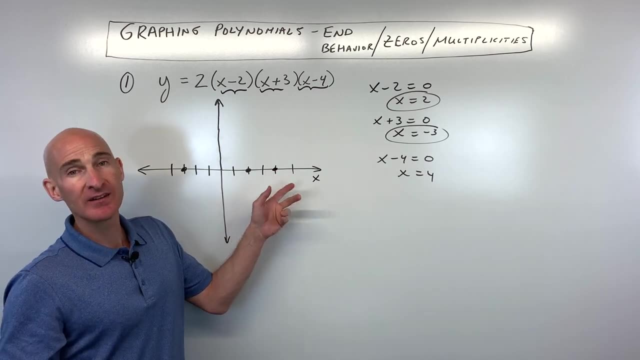 And then when you solve this last one, x equals 4, that gives us another 2.. x-intercept, or what's referred to as a zero. Now they call it a zero because the y-coordinate is zero. Basically, when you put in x equals 4, it's going to make all this zero. 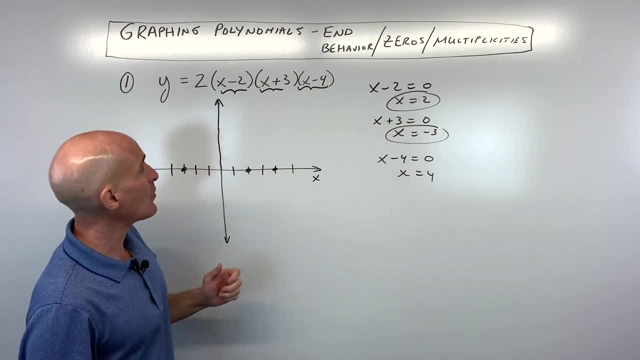 That's why the y-value is zero. We call it a zero. Now, the next thing you want to look at is: does the graph go up to the right or down to the right? Does it go up to the left or down to the left? 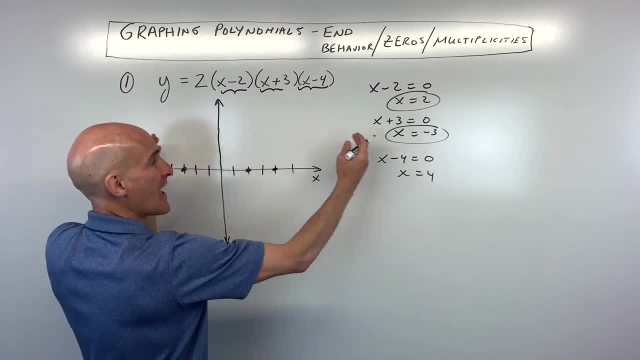 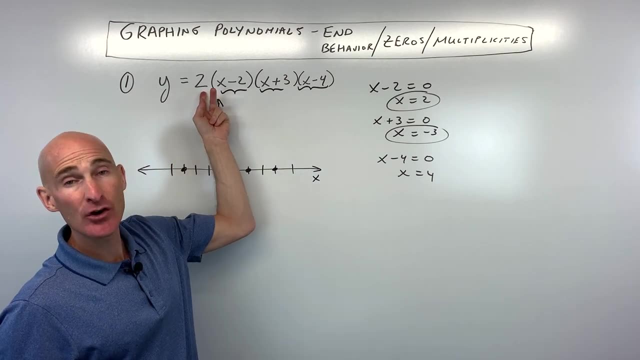 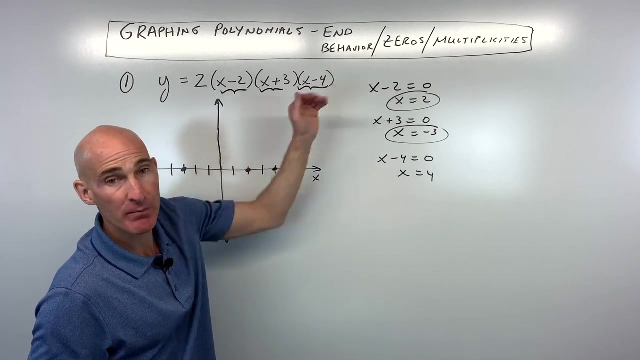 That's what it's referred to as the end behavior, meaning what happens at the ends of the graph, the left end and the right end. And the way that you determine that is by this leading coefficient. Now, the leading coefficient, if it's positive, that means it's going to go up towards positive infinity. 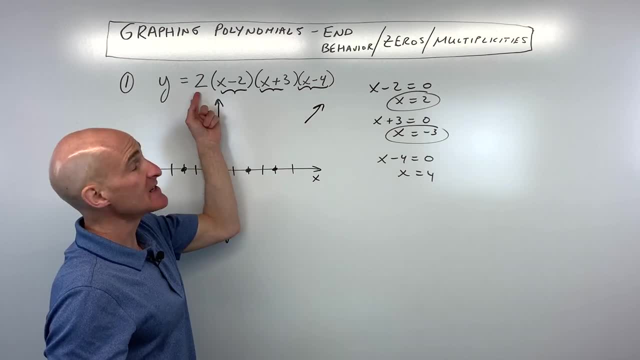 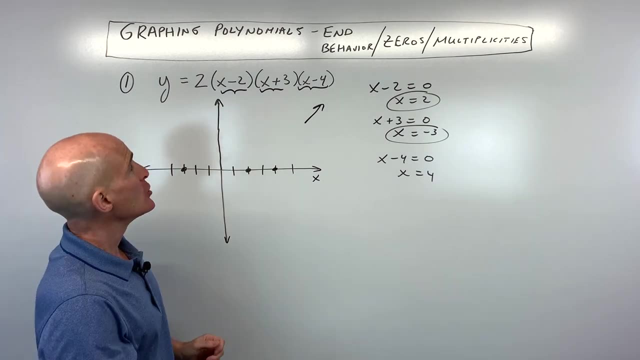 So I'm just going to draw an arrow going up to the right. If this was a negative, it's going to be going down towards negative infinity. Now, if you're not sure, you just want to test it out. you could put in a number, say, for example, like 10.. 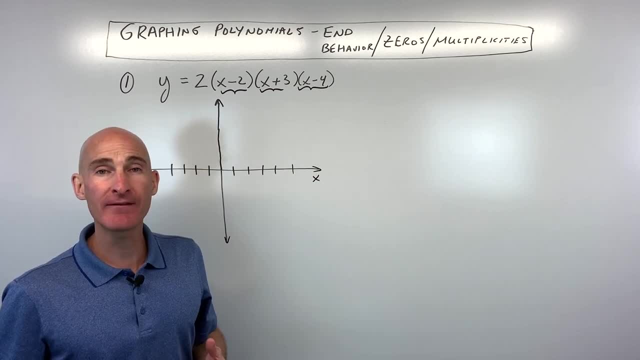 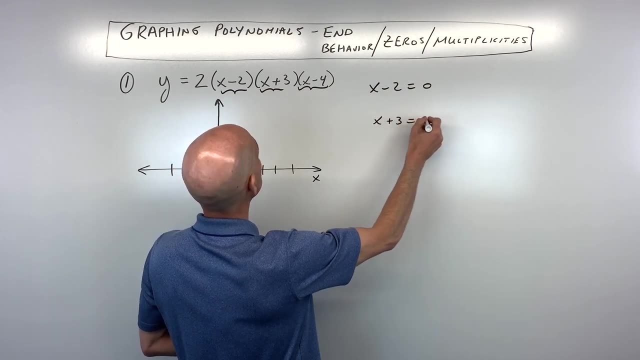 Now, if it's not factored, if you can go ahead and try and factor it, And we'll do that in the next example. So here you just make like a mini equation: x minus 2 equals 0, x plus 3 equals 0, and x minus 4 equals 0.. 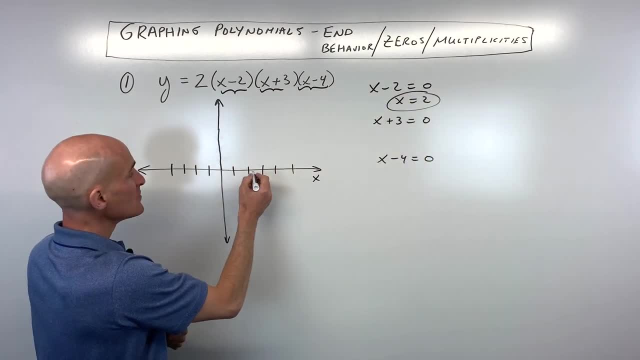 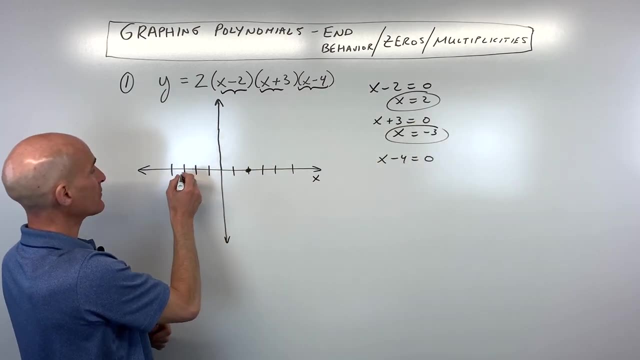 And when you solve these you can see you're getting x equals 2, which means it's going to cross the x-axis right here at 2.. Over here, when you subtract 3 from both sides, you get x equals negative 3, so it's crossing here. 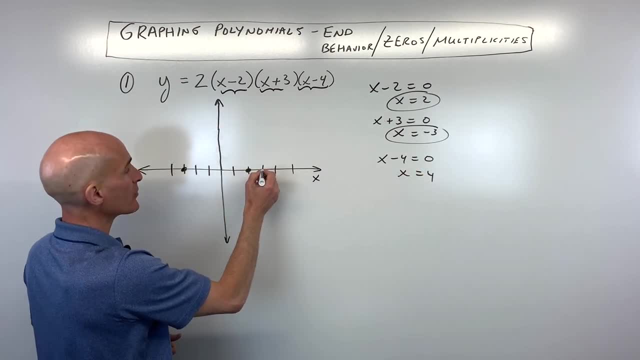 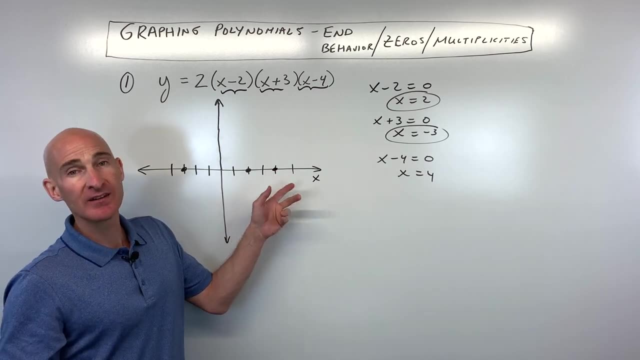 And then when you solve this last one, x equals 4, that gives us another 2.. x-intercept, or what's referred to as a zero. Now they call it a zero because the y-coordinate is zero. Basically, when you put in x equals 4, it's going to make all this zero. 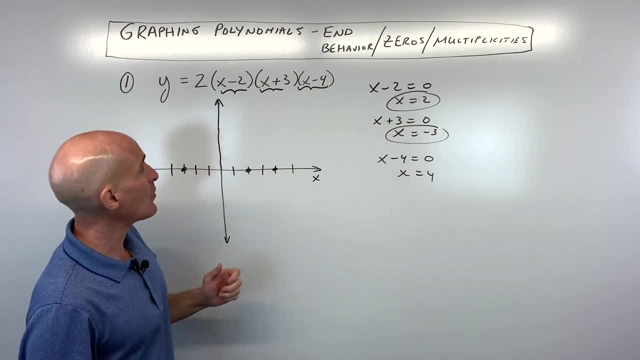 That's why the y-value is zero. We call it a zero. Now, the next thing you want to look at is: does the graph go up to the right or down to the right? Does it go up to the left or down to the left? 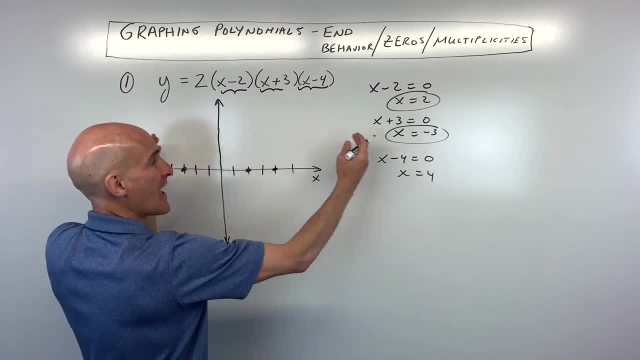 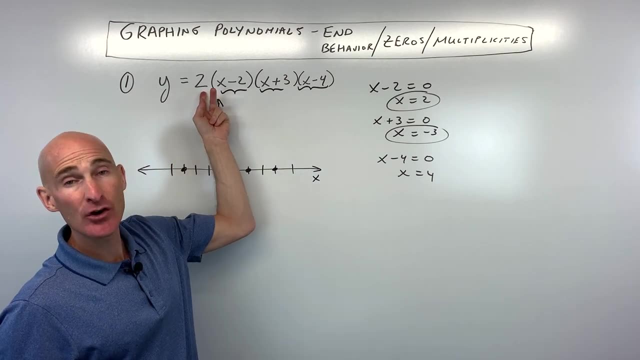 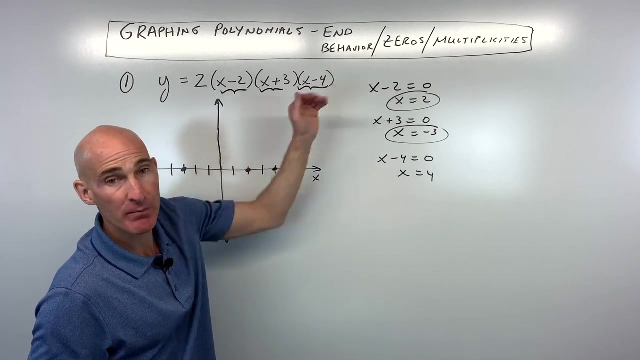 That's what it's referred to as the end behavior, meaning what happens at the ends of the graph, the left end and the right end. And the way that you determine that is by this leading coefficient. Now, the leading coefficient, if it's positive, that means it's going to go up towards positive infinity. 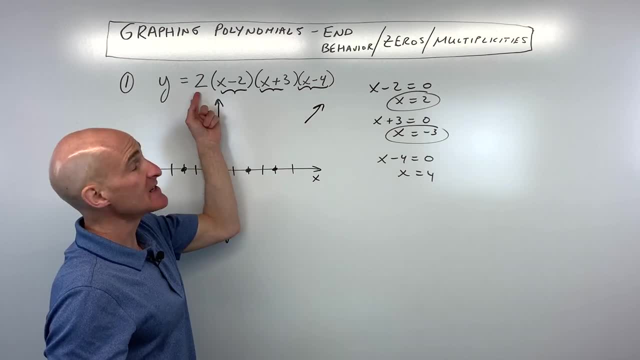 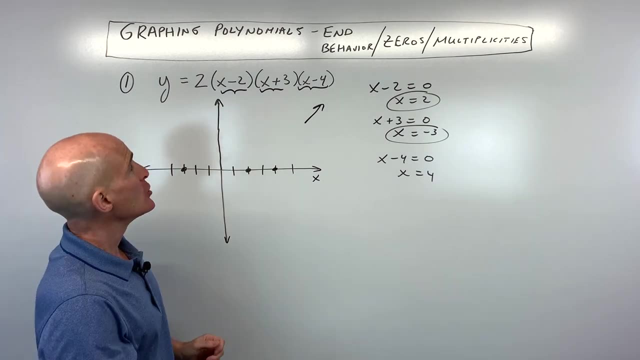 So I'm just going to draw an arrow going up to the right. If this was a negative, it's going to be going down towards negative infinity. Now, if you're not sure, you just want to test it out. you could put in a number, say, for example, like 10.. 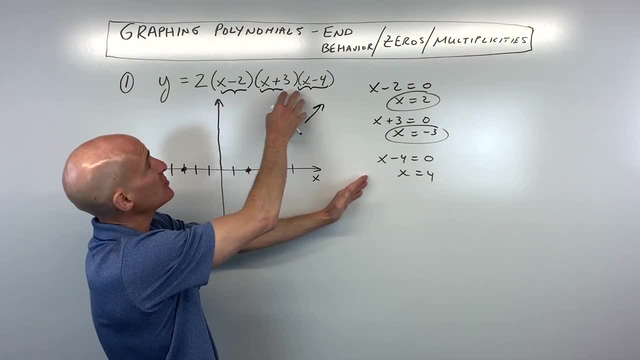 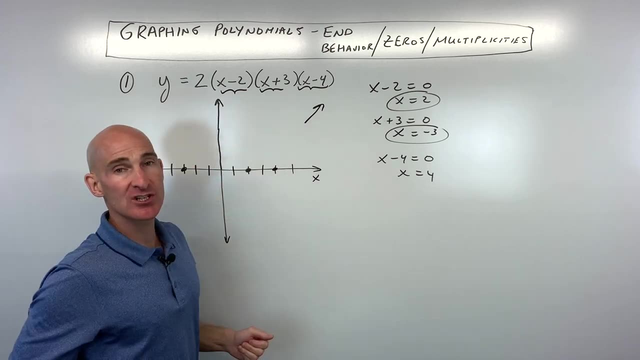 So meaning you're going way over here to the right. If you put 10 in, you're going to see that you're going to get a large positive And that tells you it's going up. but this is what's referred to as the leading coefficient test. okay or end behavior. 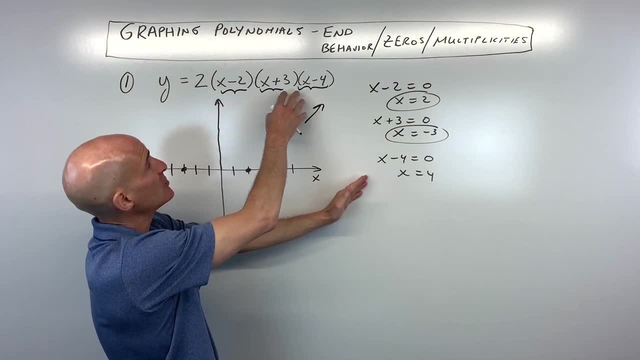 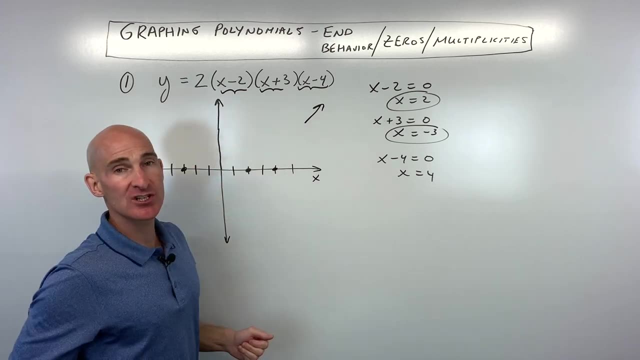 So meaning you're going way over here to the right. If you put 10 in, you're going to see that you're going to get a large positive And that tells you it's going up. But this is what's referred to as the leading coefficient test. okay or end behavior. 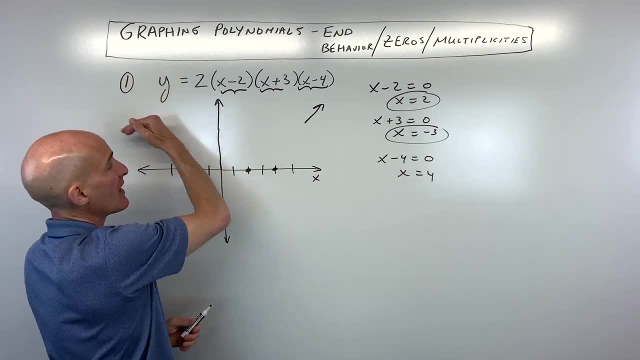 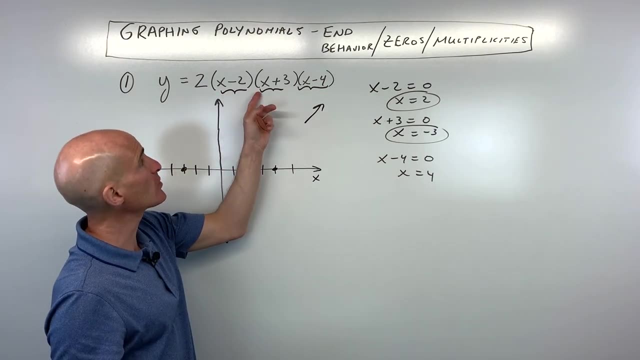 Now the next thing you want to analyze is: is the graph going up to the left or down to the left? And the way you do that is you want to look at the degree of the polynomial. What I mean by that is if you were to multiply this out, you don't have to multiply it out. 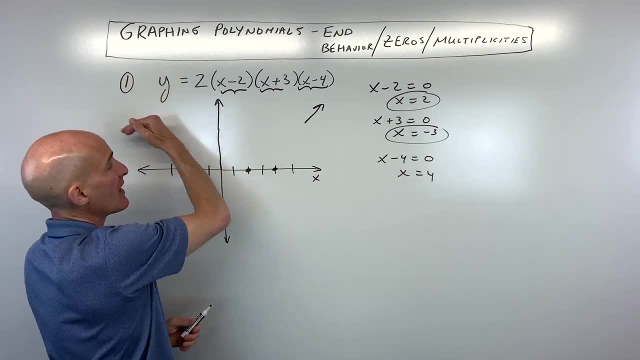 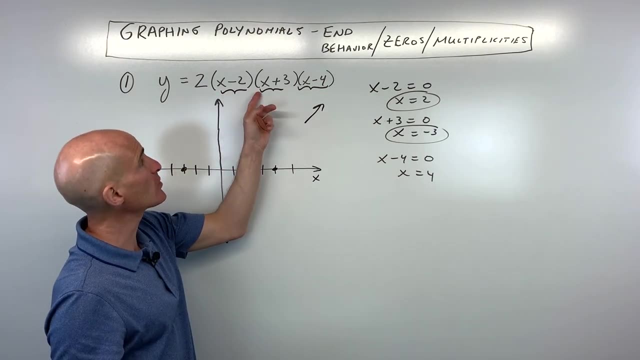 Now the next thing you want to analyze is: is the graph going up to the left or down to the left? And the way you do that is you want to look at the degree of the polynomial. What I mean by that is if you were to multiply this out, you don't have to multiply it out. 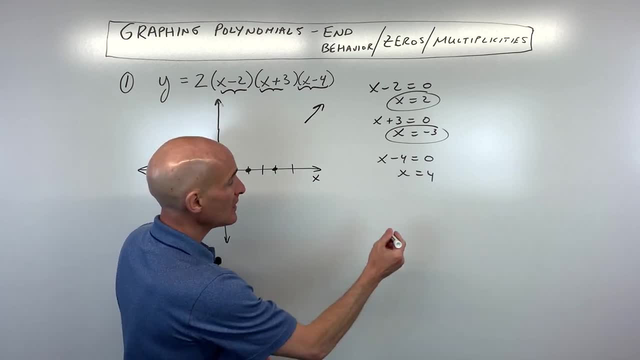 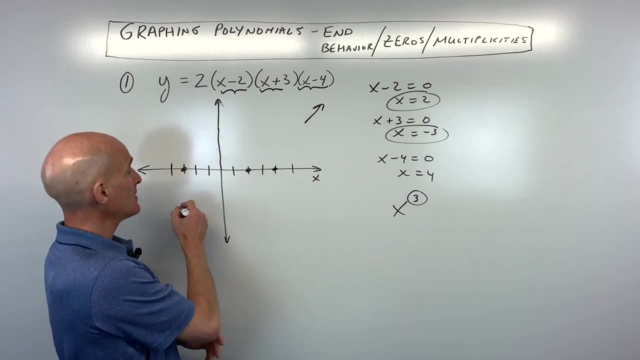 You can see it's x times x times x, which gives you x cubed, And when it's an odd degree, the end behavior- left and right- is going to be opposite, meaning: if this goes up, this goes down. If this were to go down to the right, then it would go up to the left. 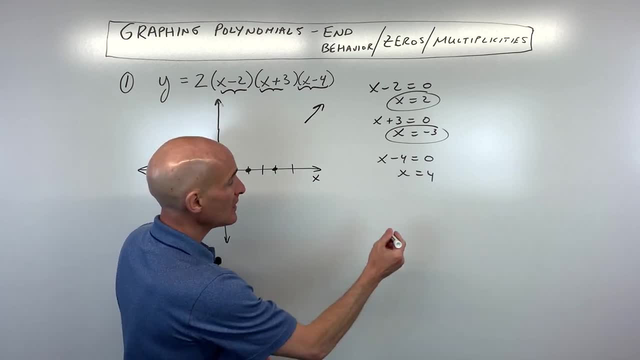 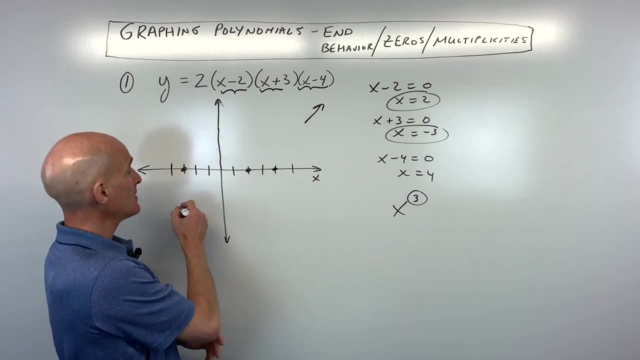 You can see it's x times x times x, which gives you x cubed, And when it's an odd degree, the end behavior- left and right- is going to be opposite Meaning: if this goes up, this goes down. If this were to go down to the right, then it would go up to the left. 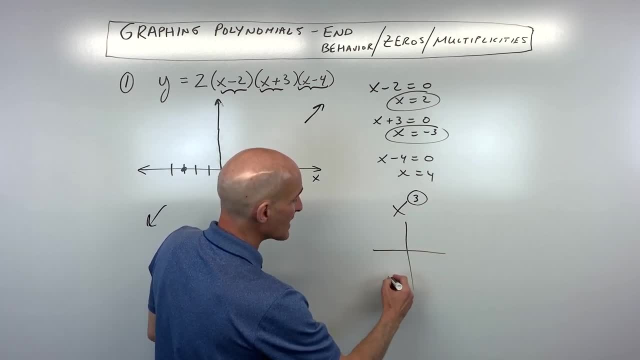 And the way you can remember that also is, if you're familiar with the graph, y equals x cubed. see how it's going up to the right and down to the left over here. If this was like a negative x cubed, it would go down to the right. 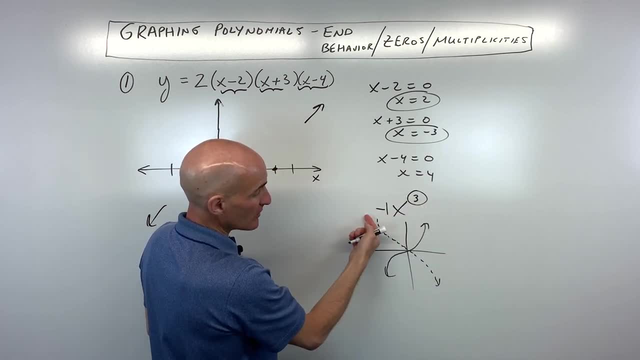 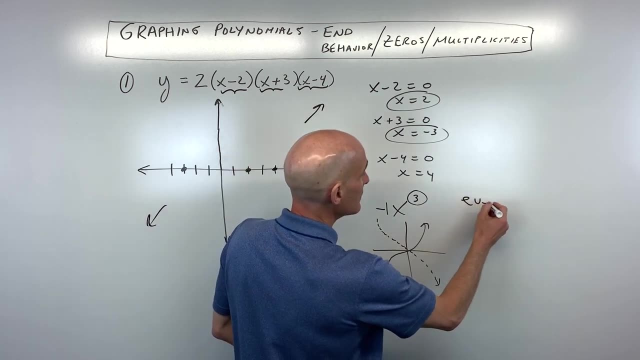 See that leading coefficient's negative one. But because it's an odd degree, it's going the opposite direction up to the left. Now, when you have an even degree, okay, even like, for example, x squared or x to the fourth. 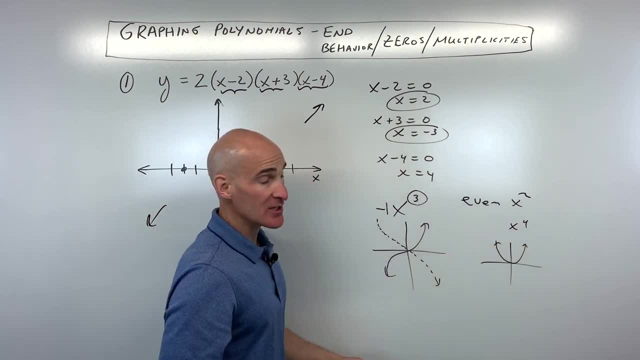 what do those graphs look like? They look like parabolas. They're either going to be both going up or, if I did- let's say I did- a negative, then you can see they're both going down. So with this even degree, it's going to have the same end behavior. 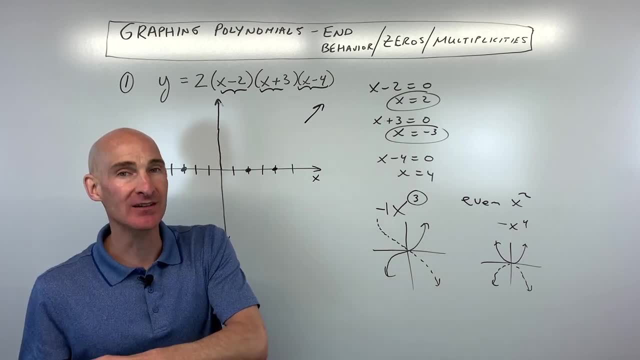 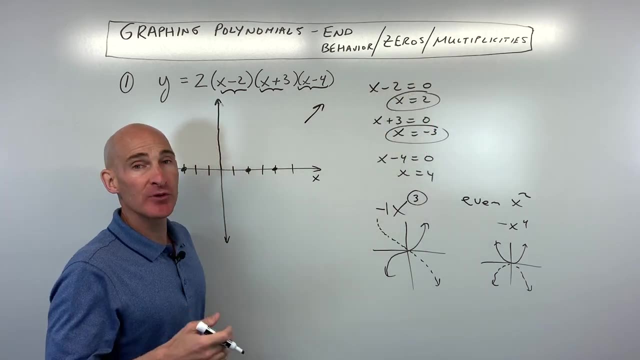 meaning both up or both down, Odd. just remember opposite O for odd, O for opposite. Easy to remember that way. Now the third thing we want to pay attention to is the multiplicities, Multiplicities. Multiplicities means like multiples, like duplicates. 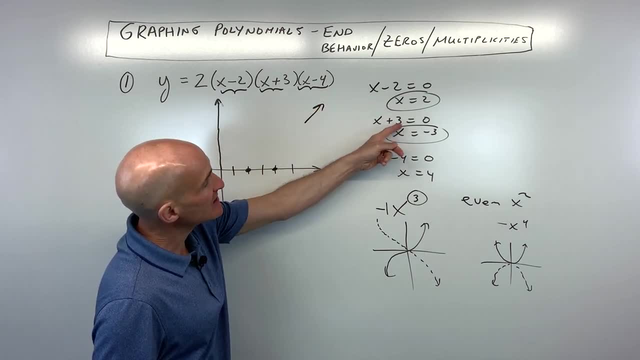 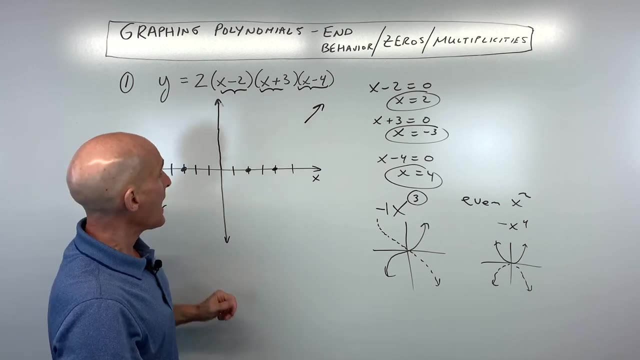 Triplicates like that, But you can see, here these did not occur more than once, We just had one, four, one negative three, one, two. When they occur just once, like that, at these zeros, at these x intercepts. 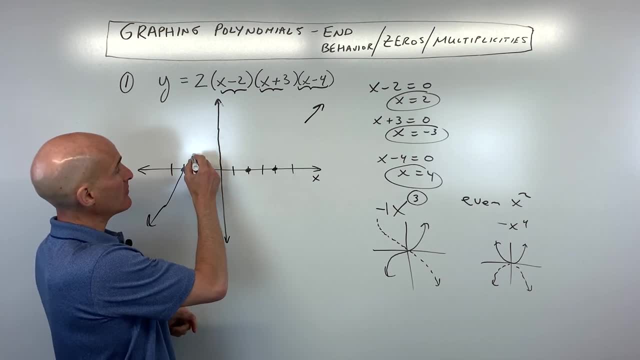 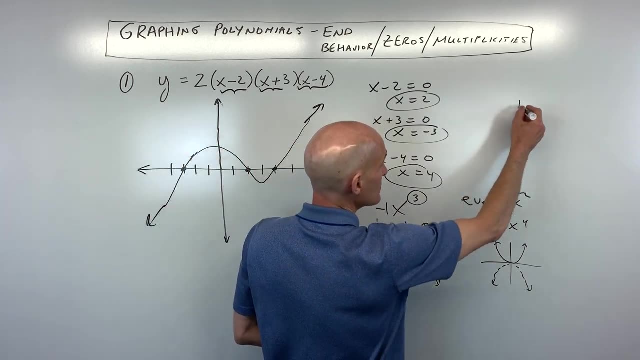 it's going to look like a line. okay, It's going to go straight through. What happens, Mario, if it occurs twice? Well, if it occurs twice, like it's a duplicate or a multiplicity of two, let's say, for example, at this point, let's say, this was two. 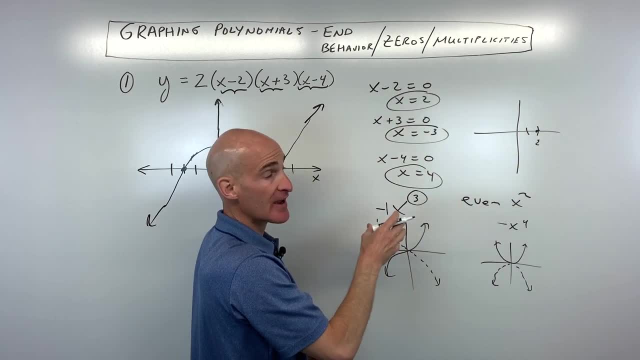 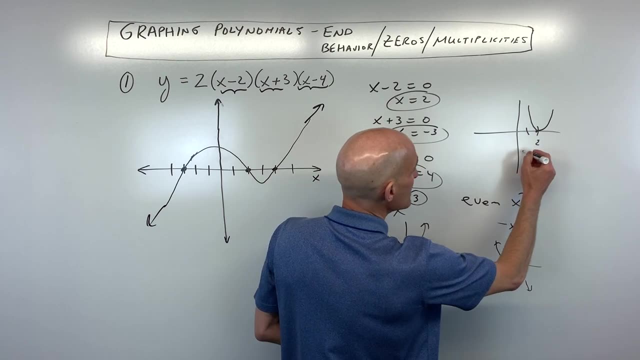 and it occurred twice, like when you factor it and you set the factors to zero, then what it has is it has a parabola shape. at that point It's going to essentially bounce off that point. If it was coming from this direction it would bounce like that. 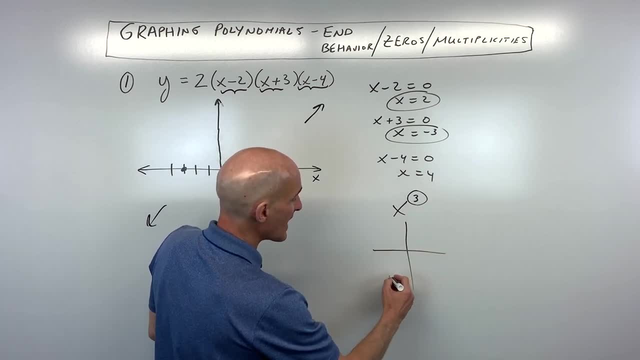 And the way you can remember that also is, if you're familiar with the graph, y equals x cubed. see how it's going up to the right and down to the left over here. If this was like a negative x cubed, it would go down to the right. 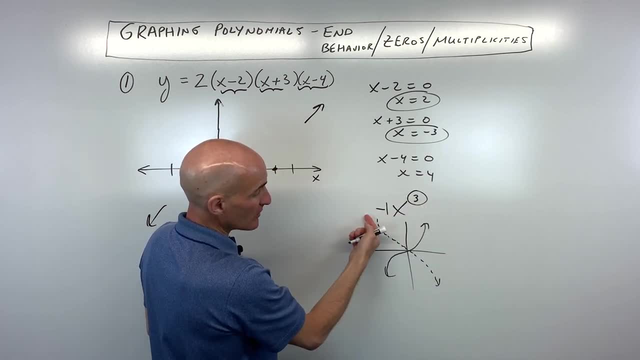 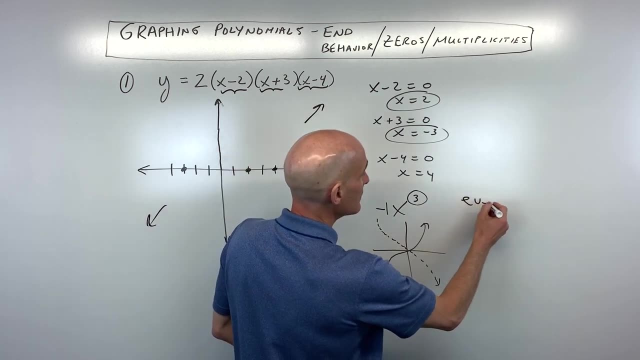 See that leading coefficient's negative 1.. But because it's an odd degree, it's going the opposite direction up to the left. Now, when you have an even degree, okay, even like, for example, x squared or x to the fourth. 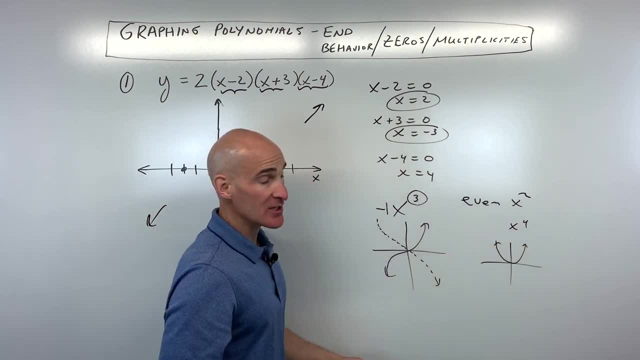 what do those graphs look like? They look like parabolas. They're either going to be both going up or, if I did- let's say I did- a negative, then you can see they're both going down. So with this even degree, it's going to have the same end behavior. 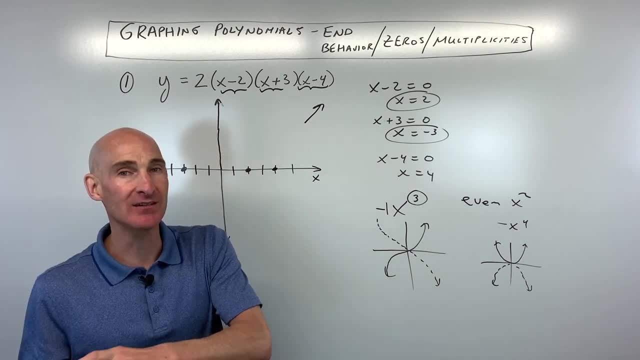 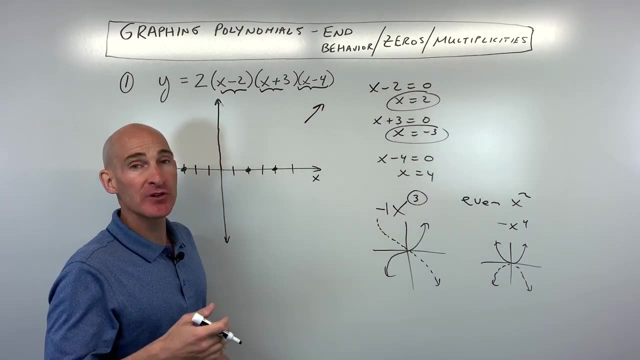 meaning both up or both down, Odd. just remember opposite O for odd, O for opposite. Easy to remember that way. Now the third thing we want to pay attention to is the multiplicities. Multiplicities means like multiples, like duplicates. 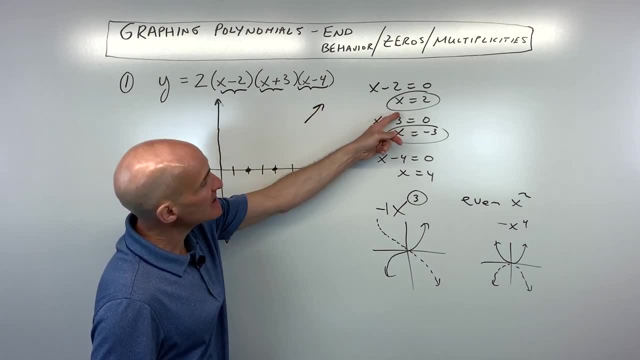 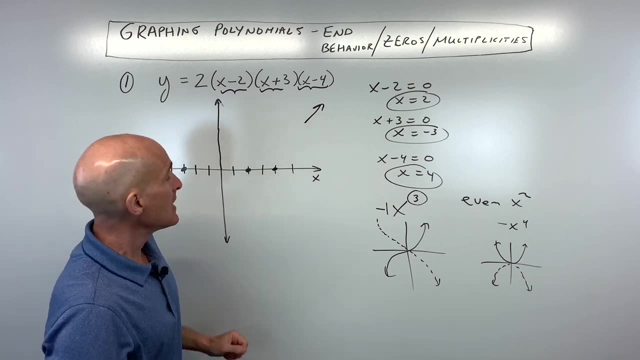 Triplicates, triplicates, like that. But you can see, here these did not occur more than once. We just had 1, 4, 1, negative 3, 1, 2.. When they occur just once, like that, at these zeros, at these x-intercepts, 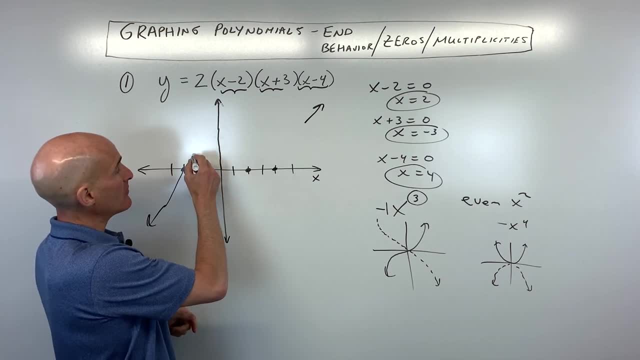 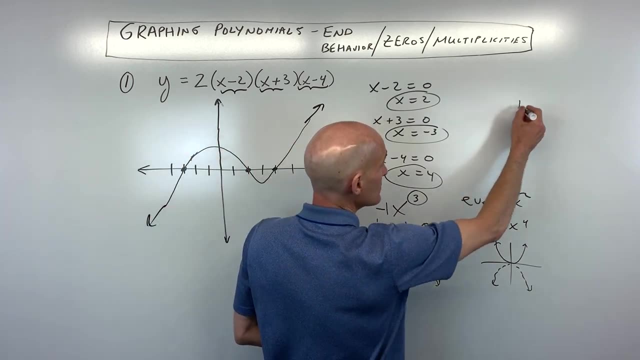 it's going to look like a line. okay, It's going to go straight through. What happens, Mario, if it occurs twice? Well, if it occurs twice, like it's a duplicate or a multiplicity of 2, let's say, for example, at this point, let's say, this was 2,. 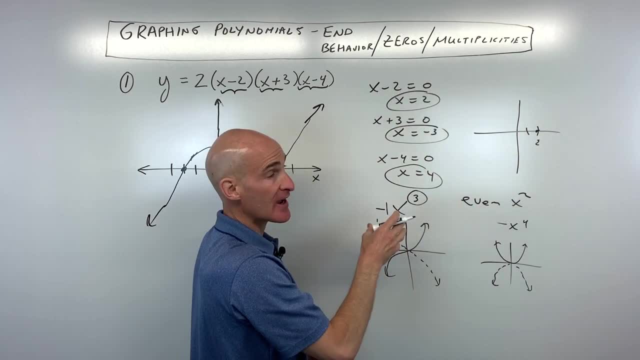 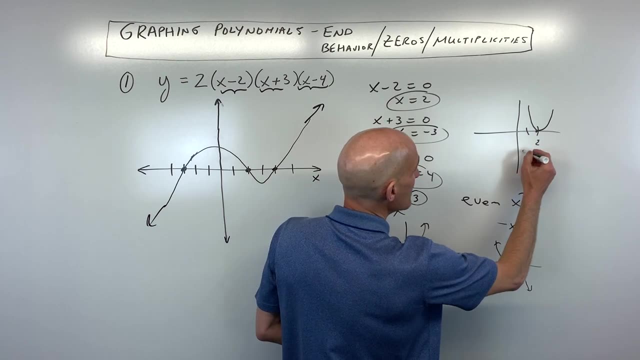 and it occurred twice, like when you factor it and you set the factors to 0, then what it has is it has a parabola shape. at that point It's going to essentially bounce off that point. If it was coming from this direction it would bounce like that. 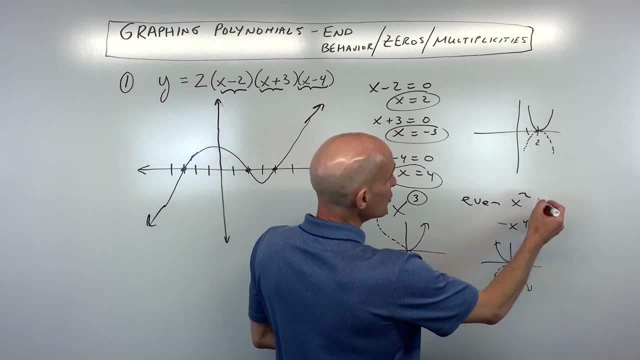 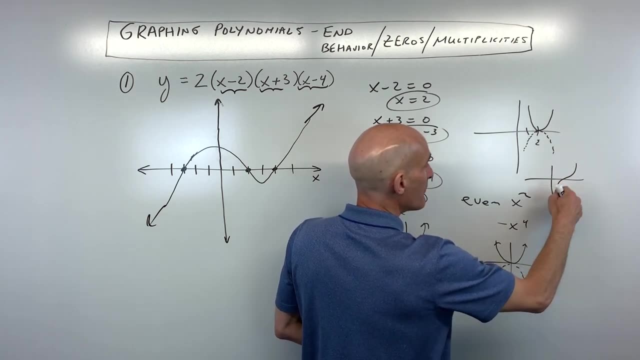 What happens if it's a multiplicity of three? Well then it's going to look like x cubed. It's going to have this x cubed shape, almost like it's going to bounce and go the other direction. Then it bends like that. 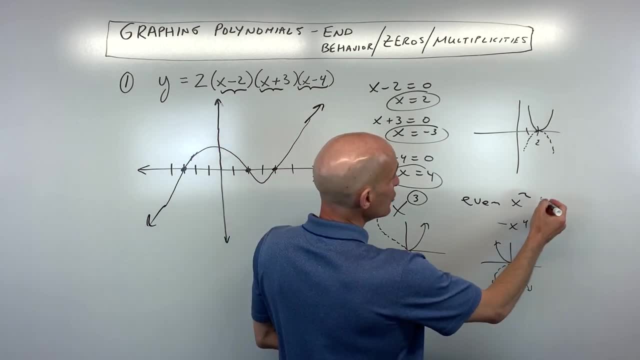 What happens if it's a multiplicity of 3?? Well then it's going to look like x-cubed. It's going to have this x-cubed shape, almost like it's going to bounce and go the other direction. 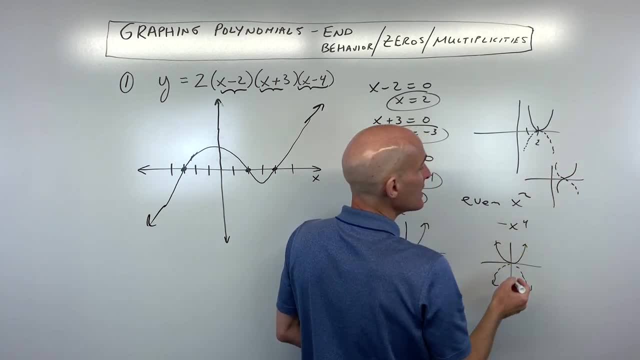 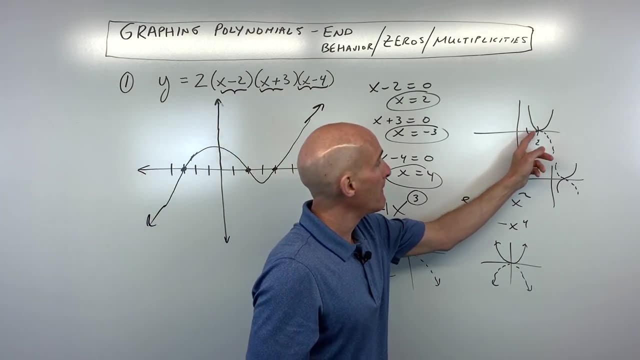 Then it bends like that. So it looks like the graph y equals x-cubed. What happens if it's x to the 4th? Well, remember if it's even. this is an easy way to remember. if it's even, it's going to bounce, okay. or look like this parabola shape: 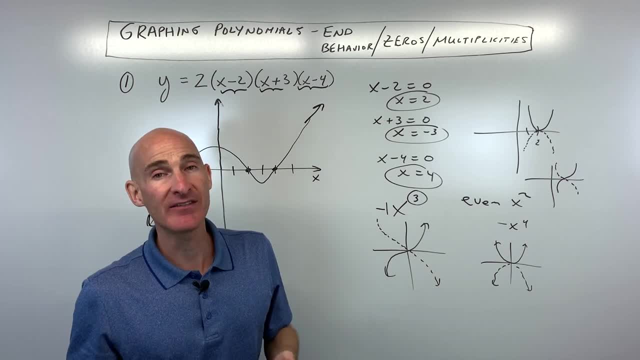 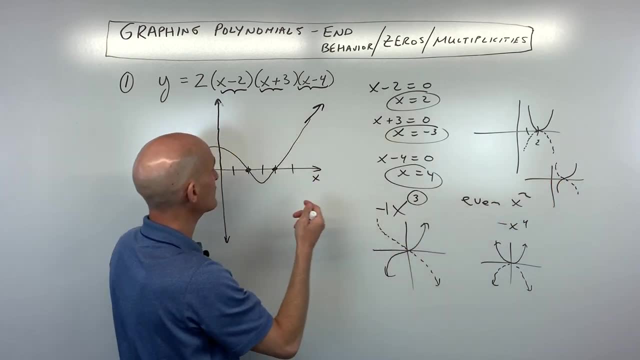 either like this or like this. If it's odd, like 1,, 3,, 5,, 7,, it's going to have this shape where it goes through, okay. And if you want to get fancy, like when it's like x-cubed or x to the 5th. 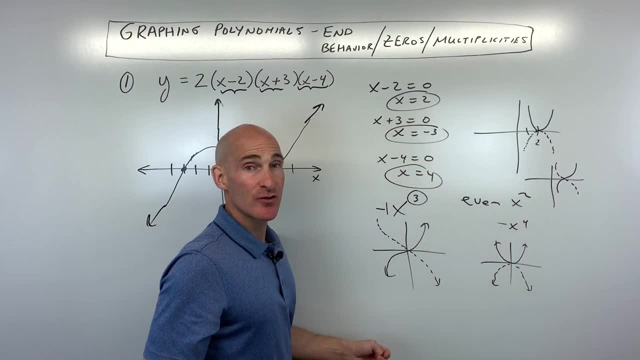 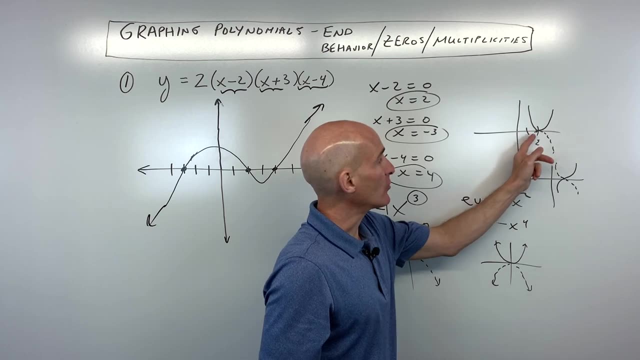 So it looks like the graph y equals x cubed. What happens if it's x to the fourth? Well, remember if it's even. this is an easy way to remember. if it's even, it's going to bounce, okay. or look like this parabola shape: 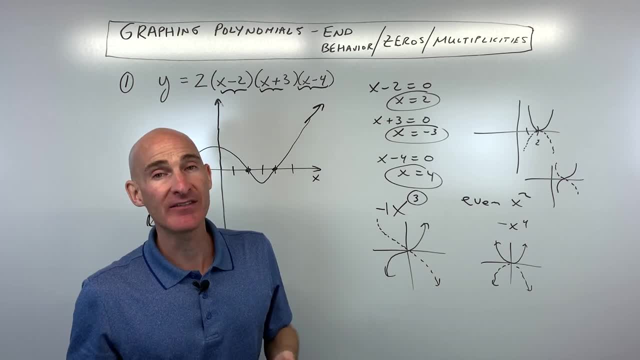 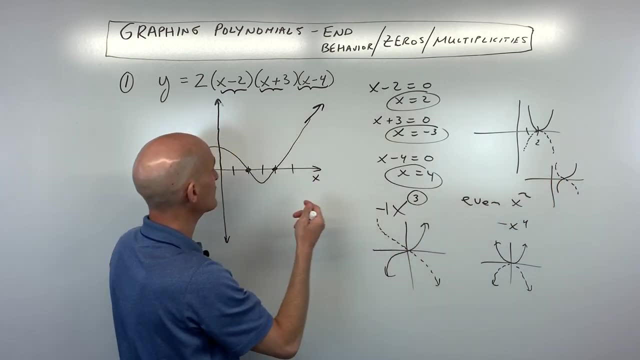 either like this or like this. If it's odd, like one, three, five, seven, it's going to have this shape, where it goes through, okay. And if you want to get fancy, like when it's like x cubed or x to the fifth. 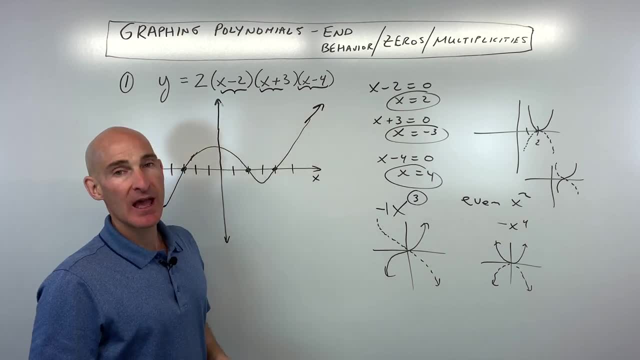 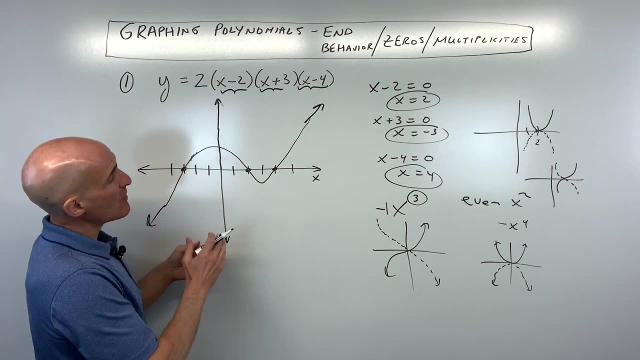 it's going to have that x cubed shape or x to the fifth shape as it passes through that point. But just remember, odd it goes through, even it doesn't, it bounces. So now the only other thing that you might be asking is you say: 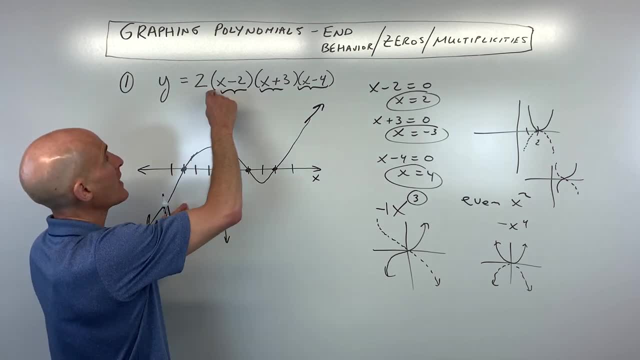 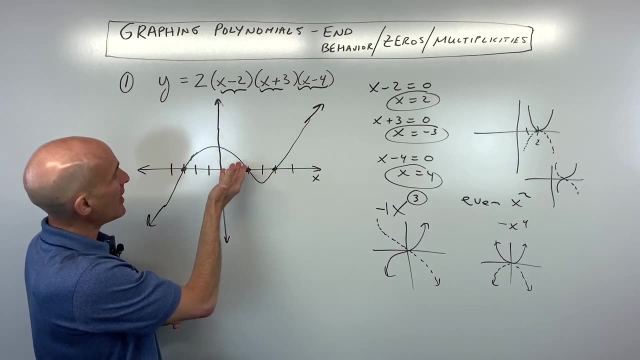 well, how did you know? like not to go way up here and then way down here and then like that? Well, you're going to learn about that. in calculus, You're going to learn about what you call the extreme values, the maximums and the minimums, these turning points or these bends. 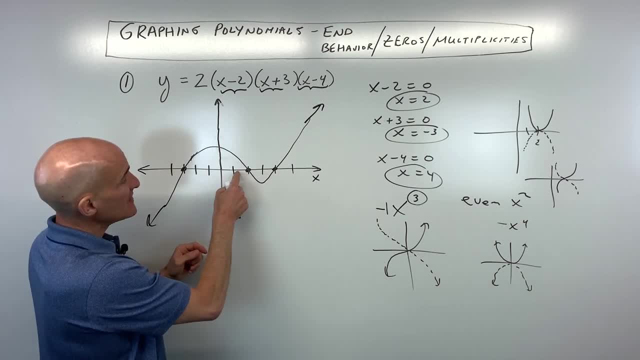 But if you want to be more precise, you could pick some points in between these x-intercepts, these zeros. You could put like three in and see what you get for the y value, or you could maybe put, like you know, negative one or negative two in. 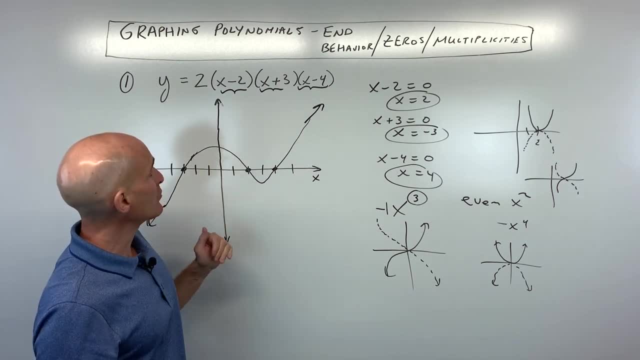 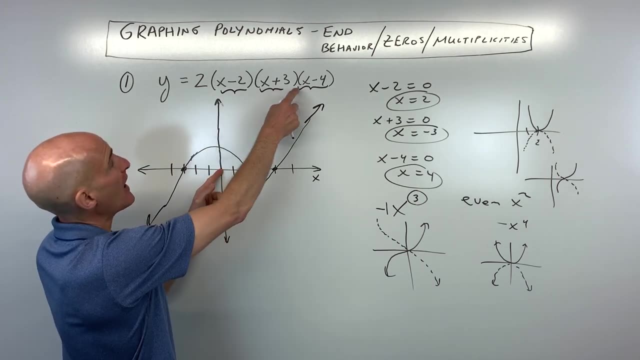 and see what you get for the y value and get a better sketch. But this is just a pretty good sketch. The key point that you might want to do is find the y-intercept. That's easy to find. You're just putting zero in for x. 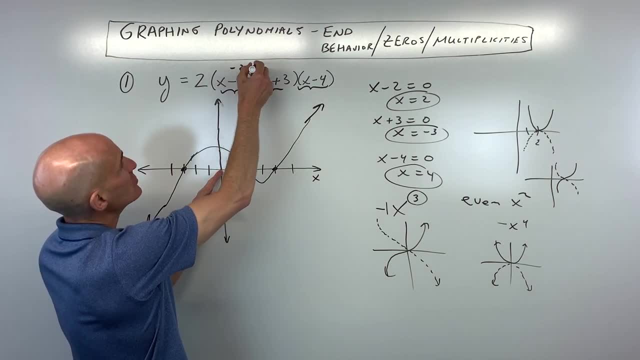 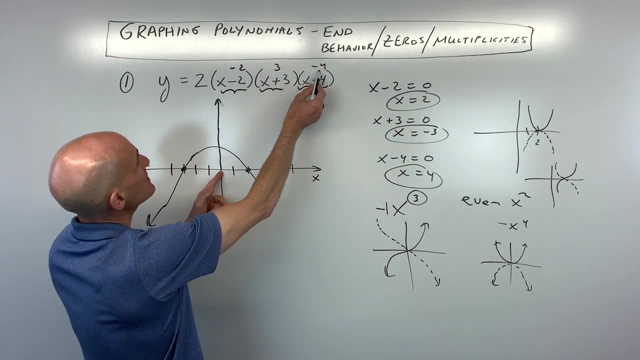 So let's go ahead and do that on this one. That would give us negative two, three and negative four, So that comes out to negative six times negative. four is twenty-four times two is forty-eight. So I really should have gone up higher. 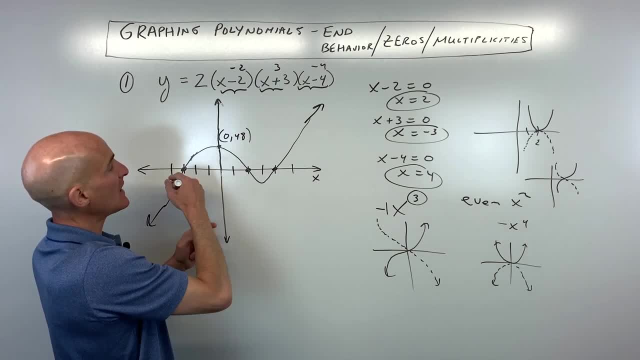 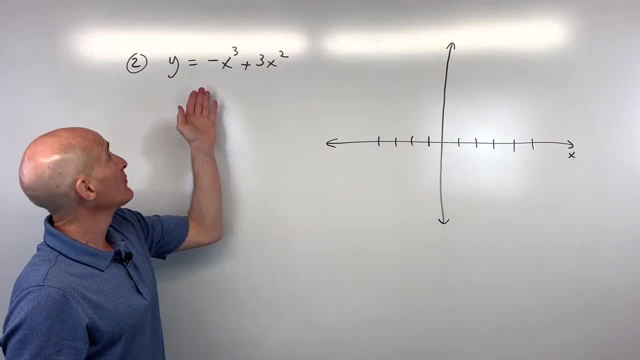 But this point here is going to be the point zero, comma forty-eight, And you have a pretty good sketch. Now let's go into some other examples to show you more about how to work with it. Okay, number two. we've got y equals negative, x cubed, plus three x squared. 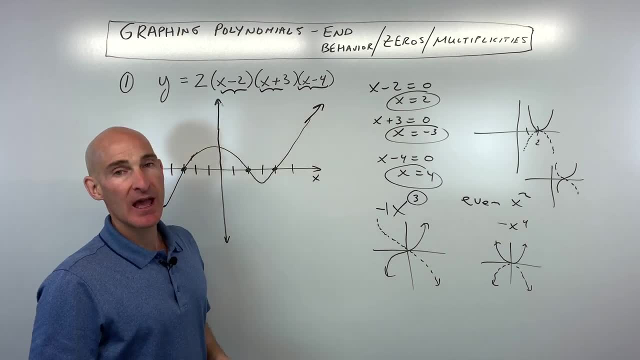 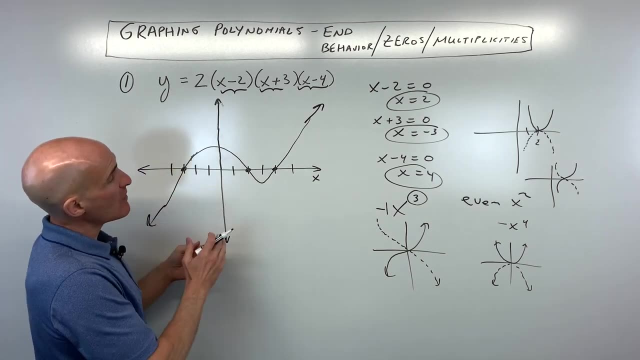 it's going to have that x-cubed shape or x to the 5th shape as it passes through that point. But just remember, odd it goes through, even it doesn't, it bounces. So now the only other thing that you might be asking is: 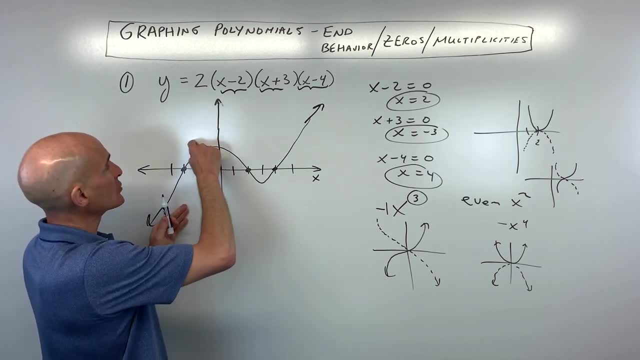 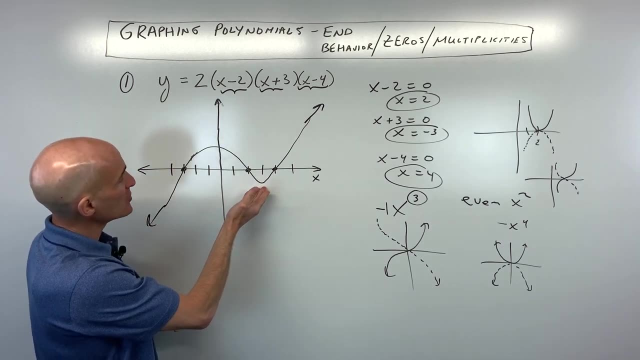 you say: well, how did you know? like not to go way up here and then way down here, and then like that. Well, you're going to learn about that. in calculus, You're going to learn about what you call the extreme values. 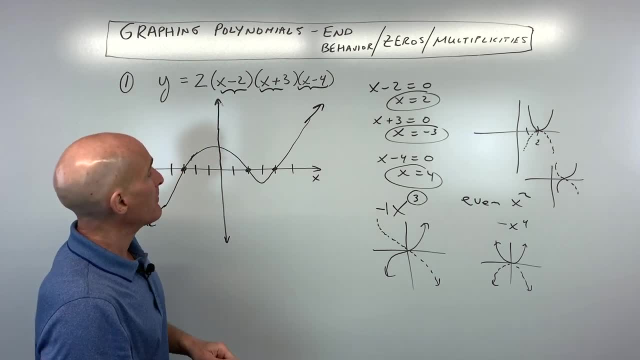 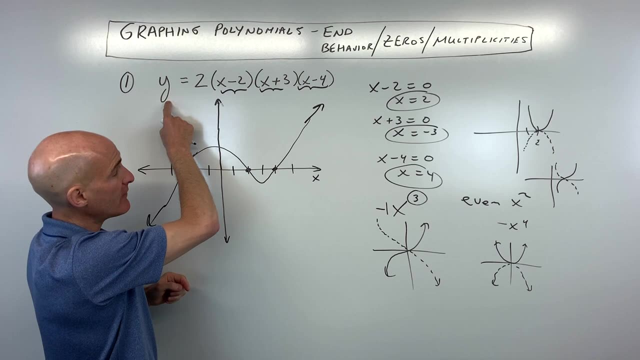 the maximums and the minimums, these turning points or these bends. But if you want to be more precise, you could pick some points in between these x-intercepts, these zeros. You could put like 3 in and see what you get for the y-value. 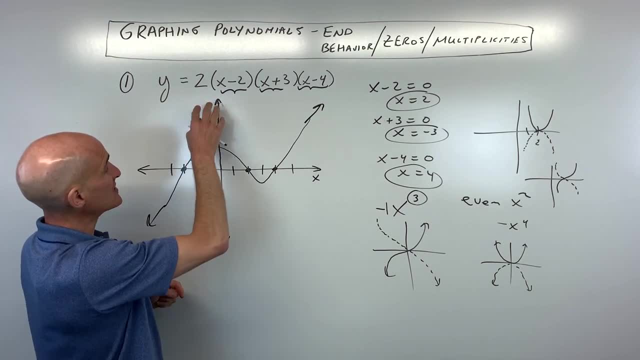 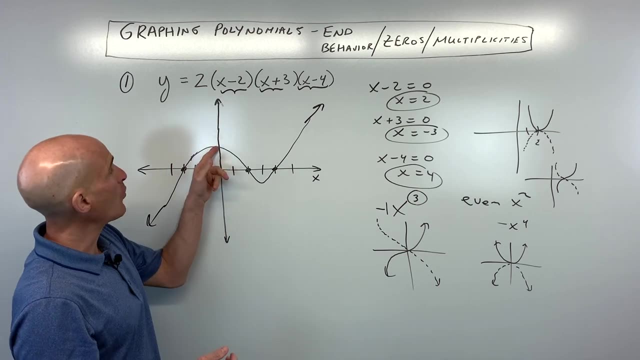 or you could maybe put, like you know, negative 1 or negative 2 in and see what you get for the y-value and get a better sketch. But this is just a pretty good sketch. One key point that you might want to do is find the y-intercept. 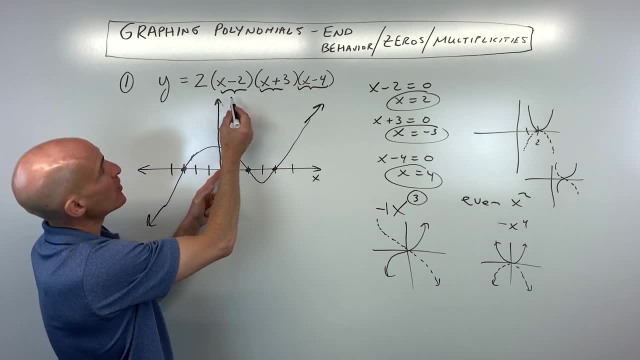 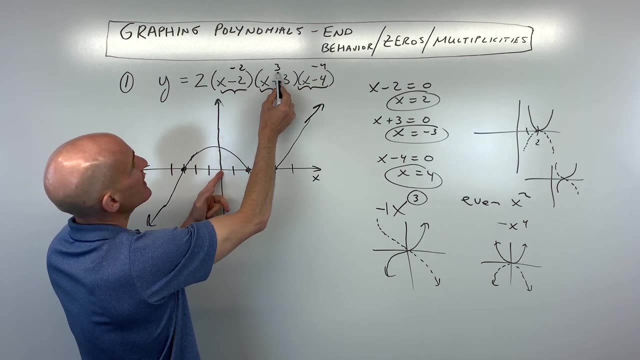 That's easy to find. You're just putting 0 in for x. So let's go ahead and do that on this one. That would give us negative 2, 3, and negative 4.. So that comes out to negative 6 times negative. 4 is 24, times 2 is 48.. 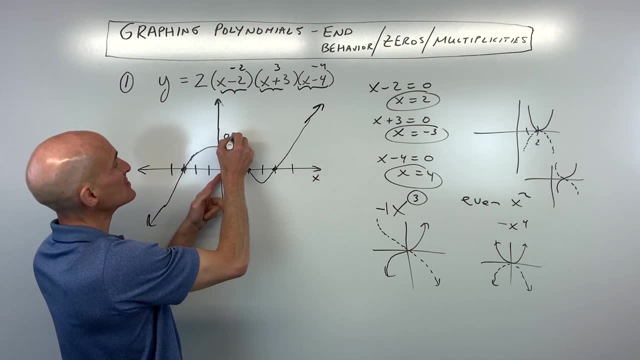 So I really should have gone up higher, but this point here is going to be the point 0, 48. And you have a pretty good sketch. Now let's go into some other examples to show you more about how to work with this. 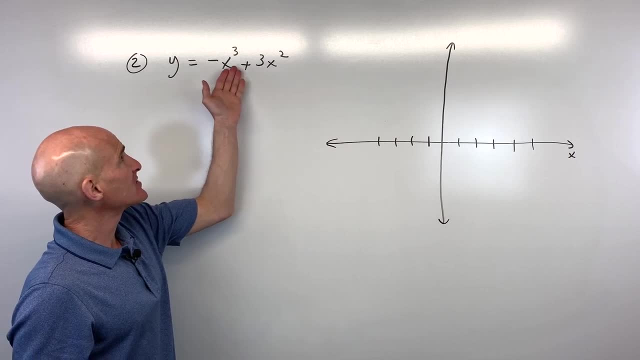 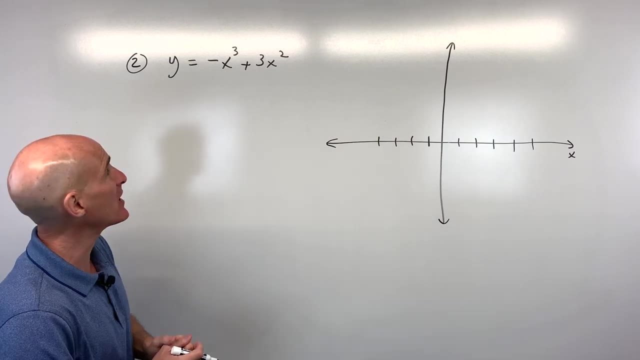 Okay, number 2, we've got y equals negative, x cubed plus 3x squared. How do we get a good graph of that using zeros and n, behavior and multiplicities? Well, the first thing you want to do, if you can, is you want to factor this: 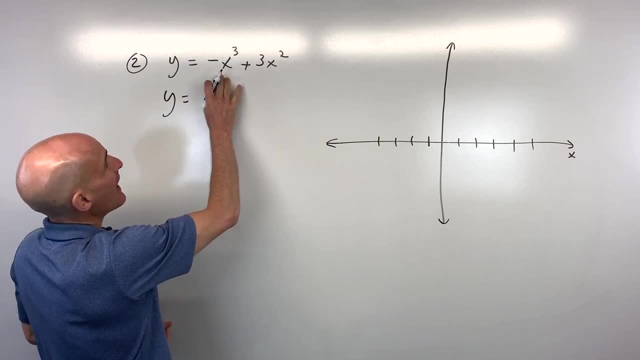 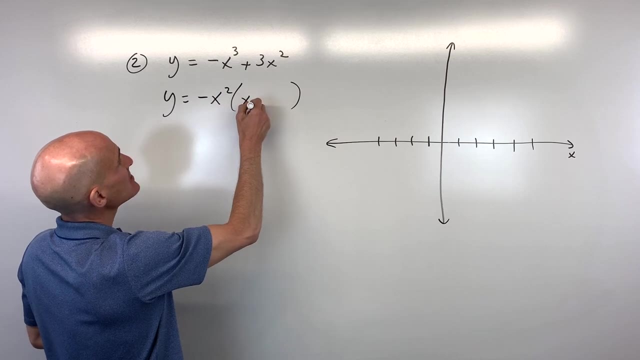 So what I notice is that I can factor out x squared, And because it starts with a negative, I'm going to factor out a negative x squared. So that's going to leave us with x minus 3.. Now you can check your work if you distribute the negative x squared back in. 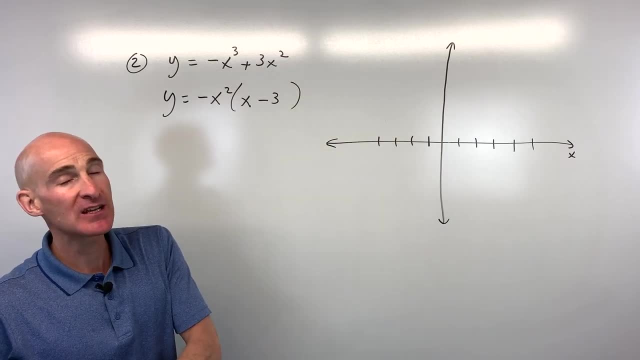 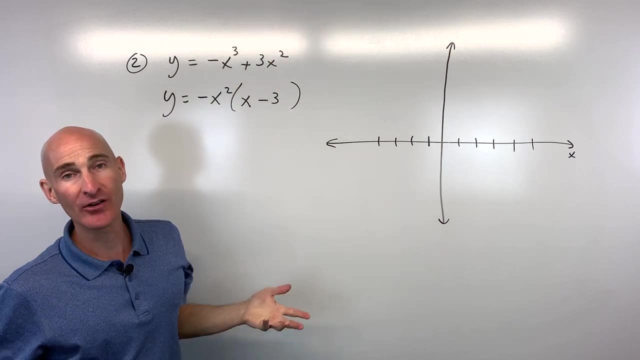 we get back the original polynomial. The other thing you want to pay attention to when you're doing this is you want to make sure you write your polynomial in descending order, So from the highest power all the way down to the lowest power. That's what standard form is, or descending order. 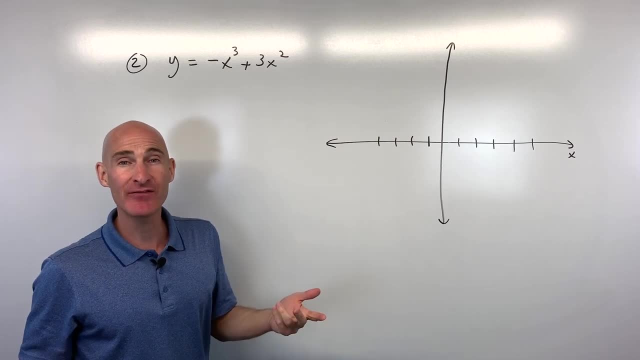 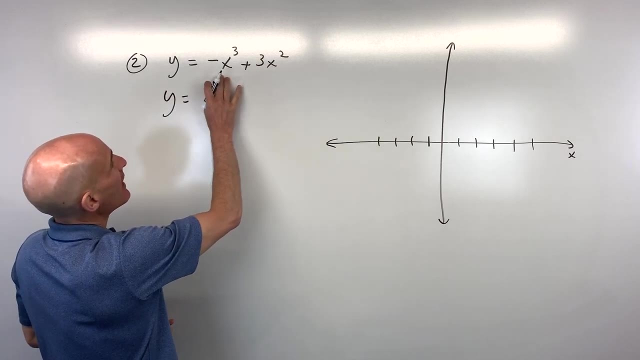 How do we get a good graph of that using zeros and n, behavior and multiplicities? Well, the first thing you want to do, if you can, is you want to factor this. So what I notice is that I can factor out x squared. 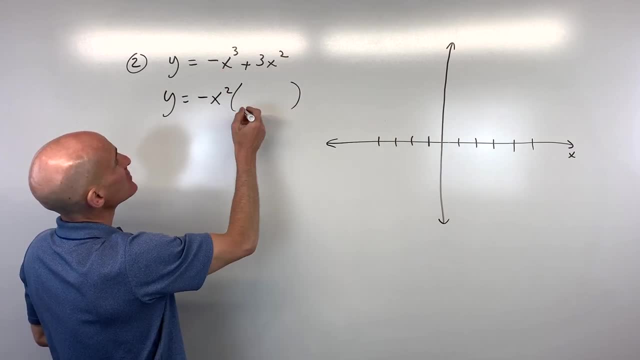 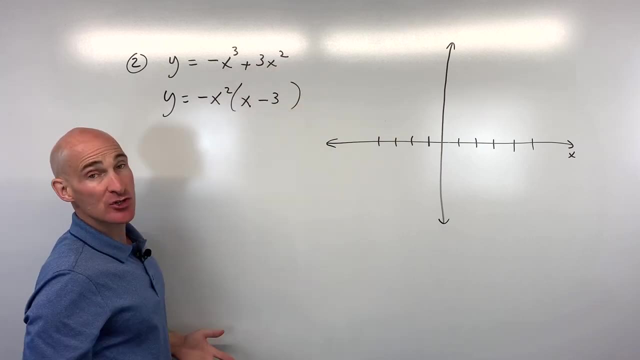 And because it starts with a negative, I'm going to factor out a negative x squared. So that's going to leave us with x minus three. Now you can check your work. if you distribute the negative x squared back in, We get back the original polynomial. 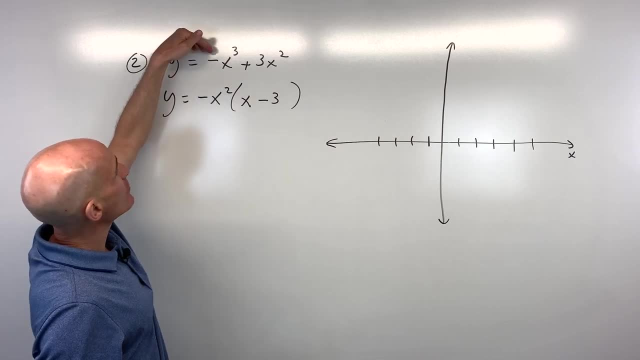 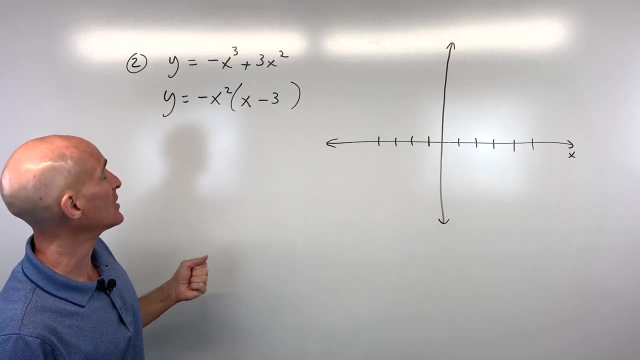 The other thing you want to pay attention to when you're doing this is you want to make sure you write your polynomial in descending order, So from the highest power all the way down to the lowest power, That's what standard form is, or descending order. 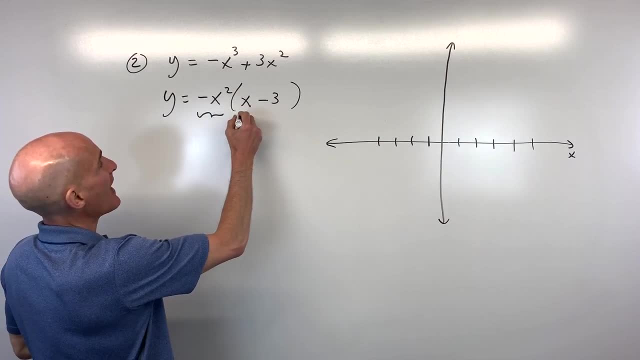 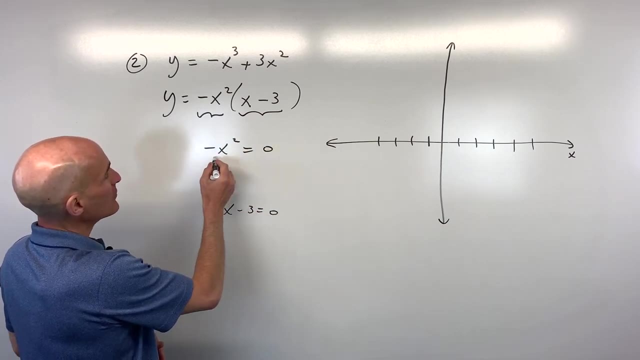 Now we have it factored. We want to set these groups or these factors equal to zero. So let's make some equations here. Negative: x squared equals zero and x minus three equals zero. If we multiply both sides by negative one, that gives us x squared equals zero. 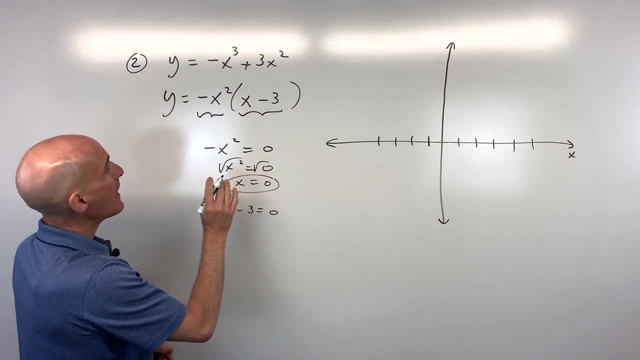 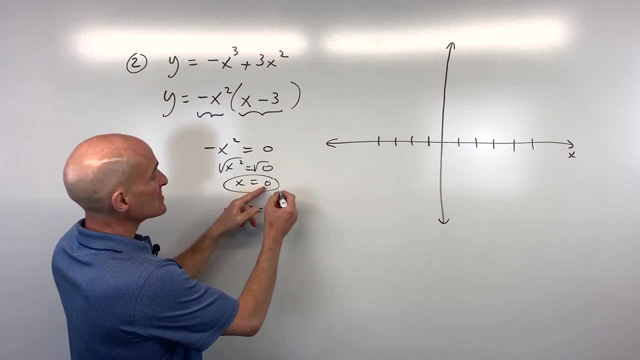 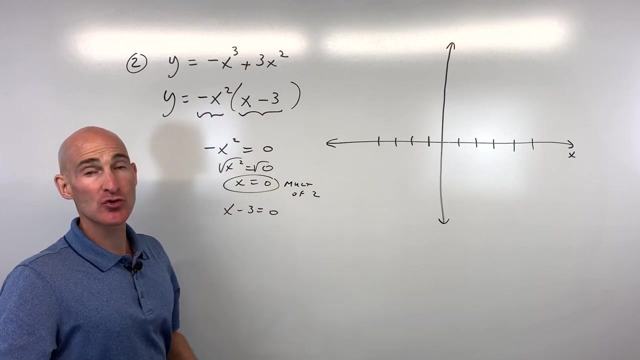 If we take the square root, okay, we're just getting zero, But you see how this is x squared, That's like x times x. We're really getting x equals zero twice. Okay, so I'm going to write this multiplicity of two, meaning it occurs twice. 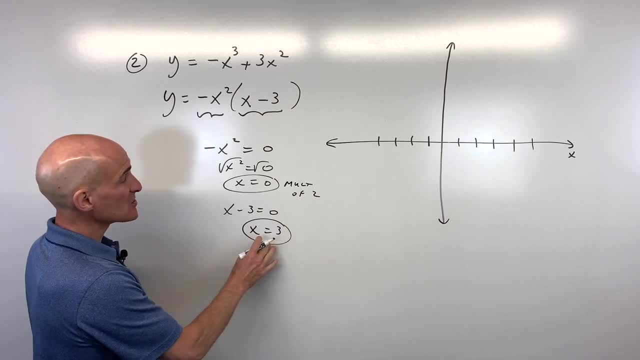 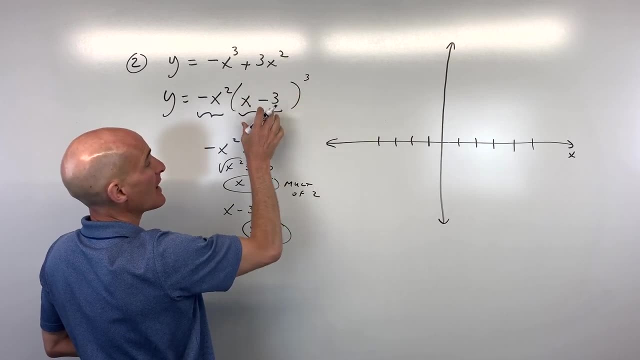 This one. when I add three to both sides, I get x equals three. This is only occurring once, So see, notice, this is x squared. If I had like a three here, like x minus three cubed, then I would have three, three times. 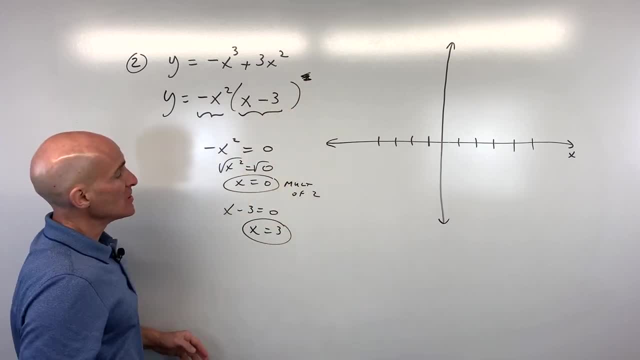 That would be like a multiplicity of three, But this only occurs once, So I'm going to write this multiplicity of three times. So now what we're going to do is we're going to plot that on our x-axis. These are our zeros, or our x-intercepts. 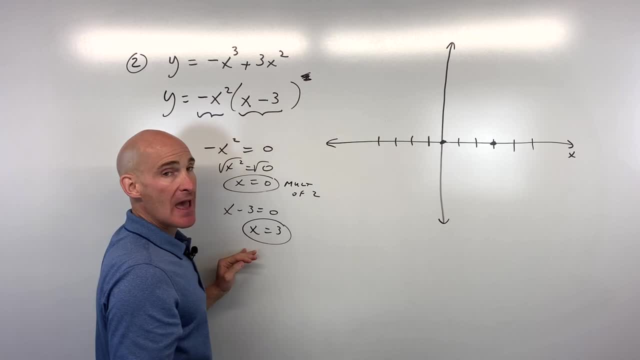 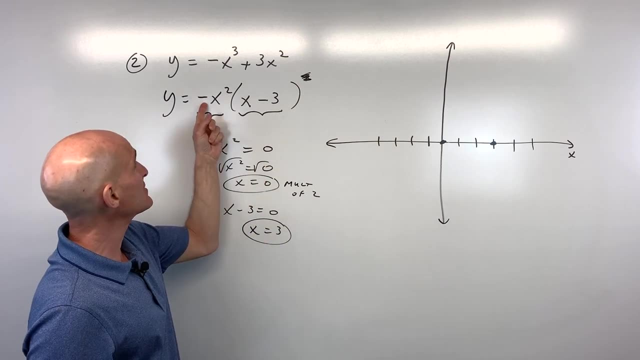 We've got zero and three. Let's go to n behavior now. So do you think the graph is going to go up to the right or down to the right? What do you think? Well, if you said down to the right, you're absolutely right, because it has that leading coefficient which is negative. 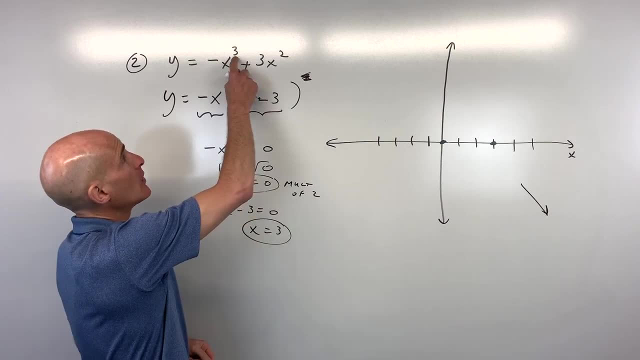 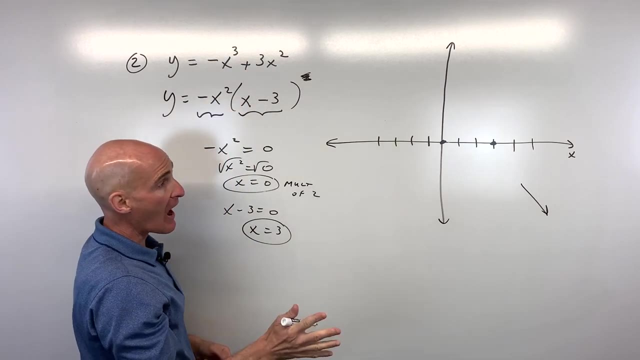 And then, what about for the left-hand behavior? Is it going up or down? Well, the degree, okay. when we talk about degree, that's the highest power here, which is three. that's odd. Remember, odd is opposite. 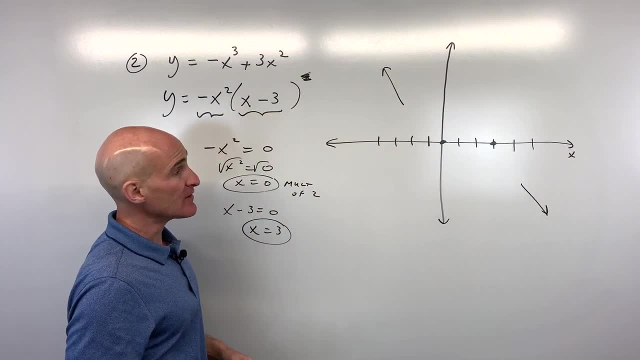 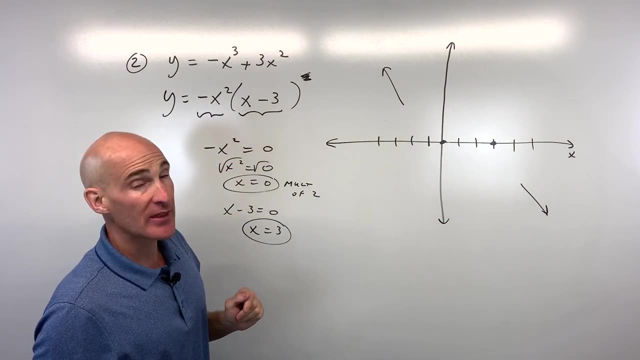 So we're going up to the left. If it's even degree, like if this is x to the fourth, then these would be the same, either both down or both up. So now we have to look at the multiplicities. We said that zero occurs twice. 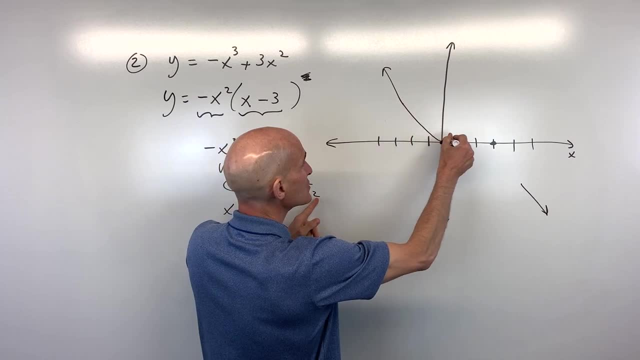 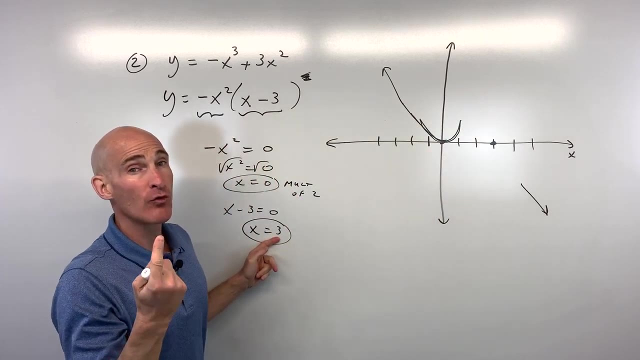 So here at x equals zero, because it occurs twice, it's going to look like a parabola, like x squared Okay. so it's going to have this kind of a shape Over here: x equals three. this only has a multiplicity of one. 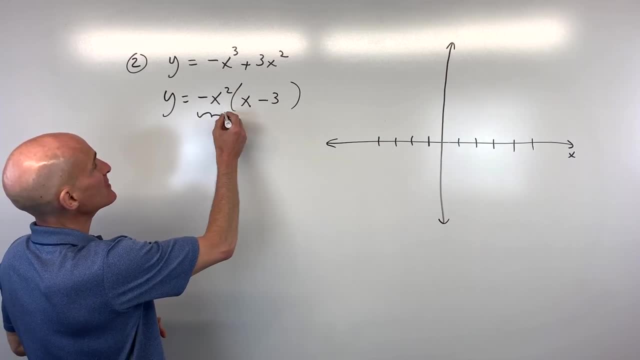 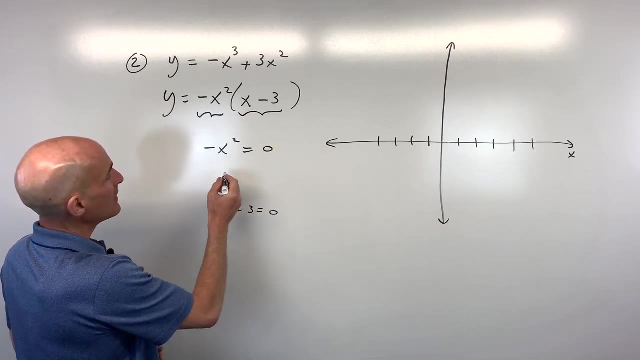 Now we have it factored, We want to set these groups or these factors equal to 0.. So let's make some equations here. Negative x squared equals 0, and x minus 3 equals 0. If we multiply both sides by negative 1,, that gives us x squared equals 0.. 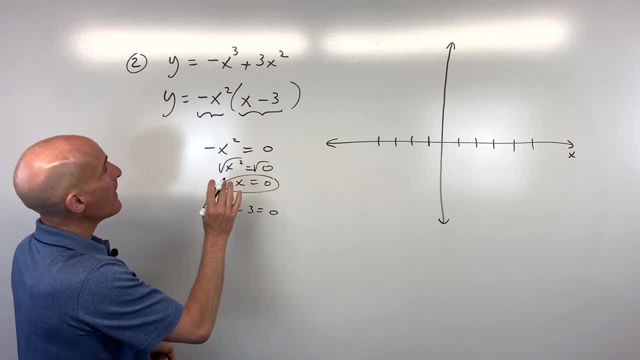 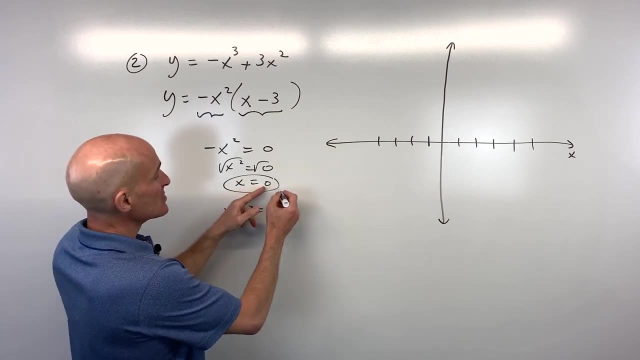 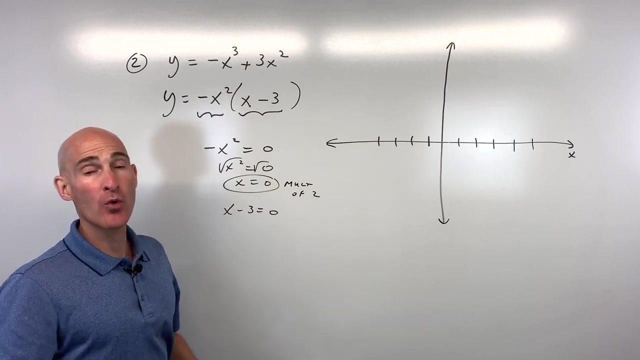 If we take the square root, okay, we're just getting 0.. But you see how this is x squared. That's like x times x. We're really getting x equals 0 twice. Okay. so I'm going to write this multiplicity of 2, meaning it occurs twice. 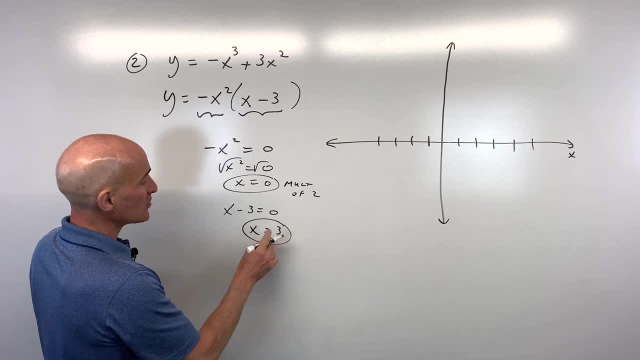 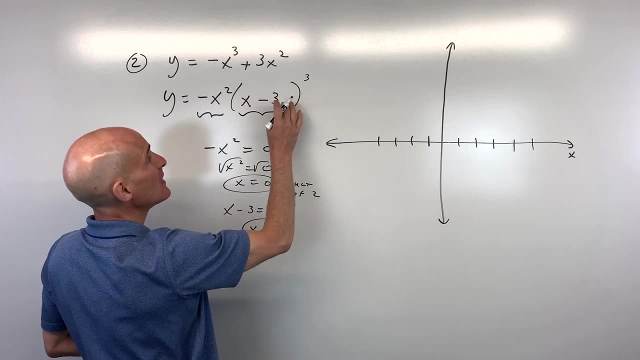 This one. when I add 3 to both sides, I get x equals 3.. This is only occurring once, So see notice: this is x squared. If I had like a 3 here, like x minus 3 cubed, then I would have 3, 3 times. 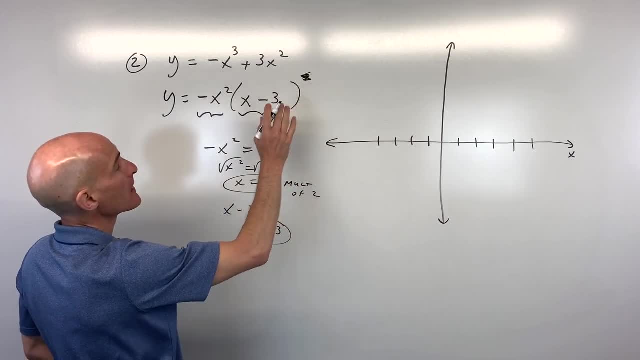 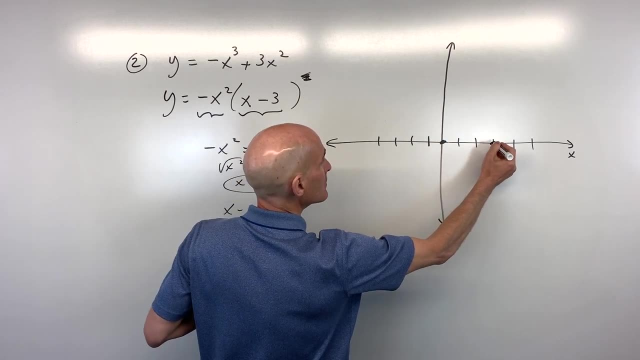 That would be like a multiplicity of 3.. But this only occurs once here. So now what we're going to do is we're going to plot that on our x-axis. These are our zeros, or our x-intercepts. We've got 0 and 3.. 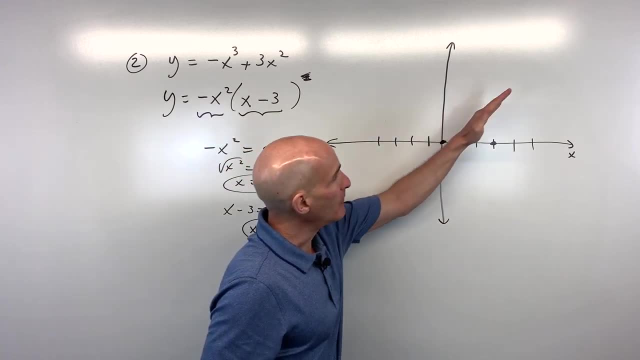 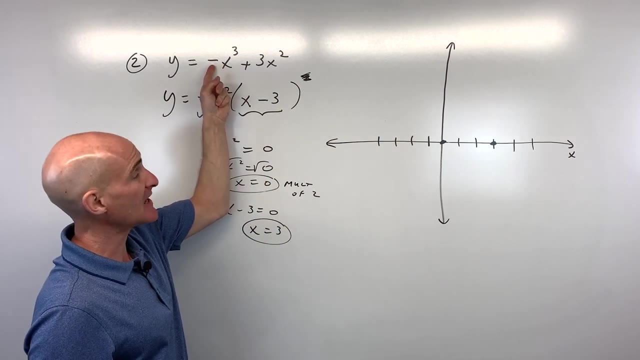 Let's go to n behavior now. So do you think the graph is going to go up to the right or down to the right? What do you think? Well, if you said down to the right, you're absolutely right, because it has that leading coefficient which is negative. 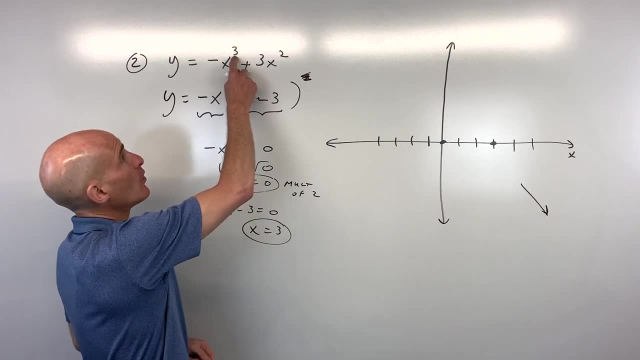 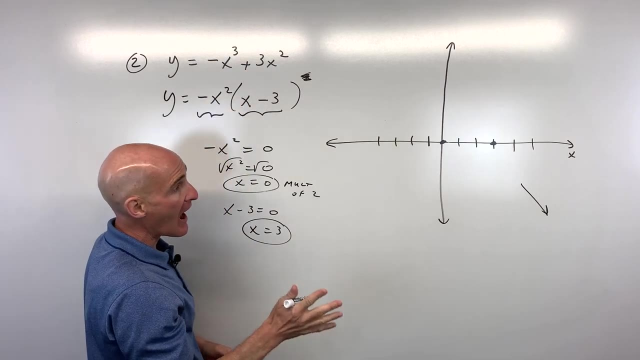 And then, what about for the left-hand behavior? Is it going up or down? Well, the degree, okay. when we talk about degree, that's the highest power here, which is 3.. That's odd, Remember, odd is opposite. 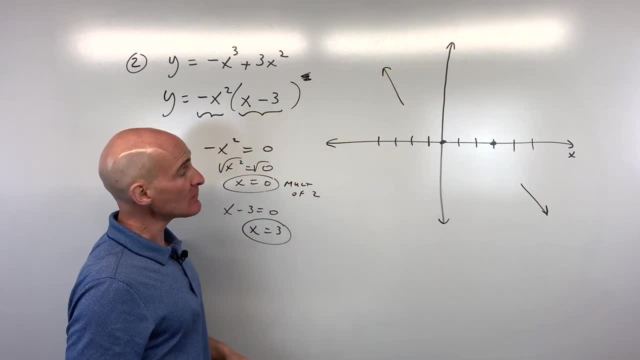 So we're going up to the left. If it's even degree, like if this is x to the fourth, then these would be the same, either both down or both up. So now we have to look at the multiplicities. We said that 0 occurs twice. 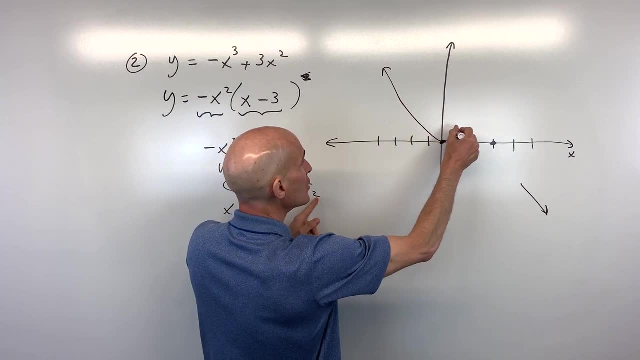 So here at x equals 0, because it occurs twice, it's going to look like a parabola, like x squared Okay. so it's going to have this kind of a shape Over here: x equals 3, this only has a multiplicity of 1.. 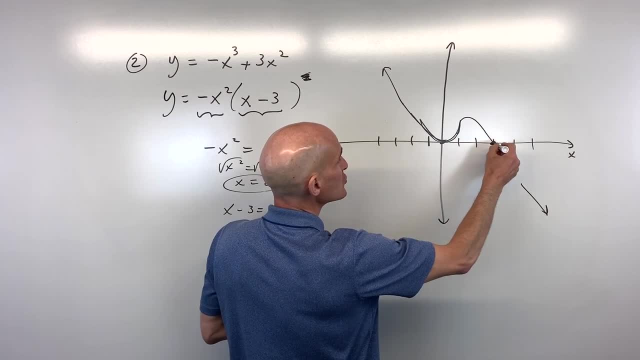 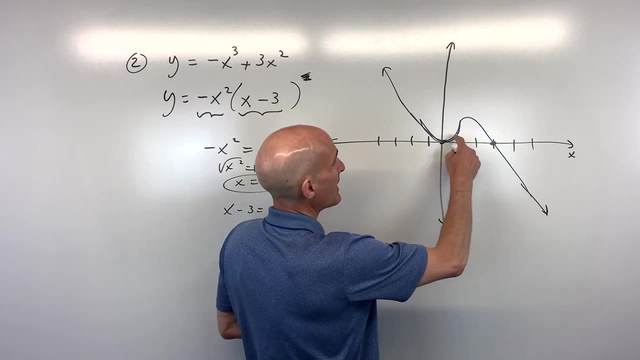 It just occurs once. That means this is going to just go straight through like a line. okay. So the only thing is, you know you might be saying: how did I not go all the way up here, right? Or how come I didn't just go like that? 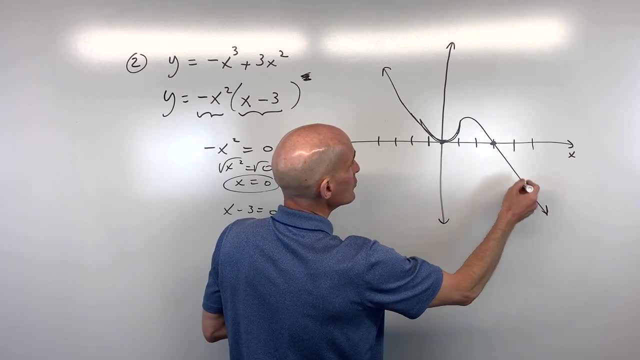 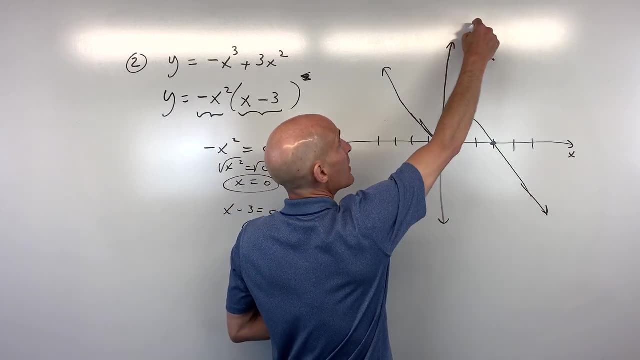 It just occurs once. That means this is going to be x squared. Okay, so it's going to have this kind of a shape. It's going to just go straight through like a line, Okay. so the only thing is, you know, you might be saying: how did I not go all the way up here, right? 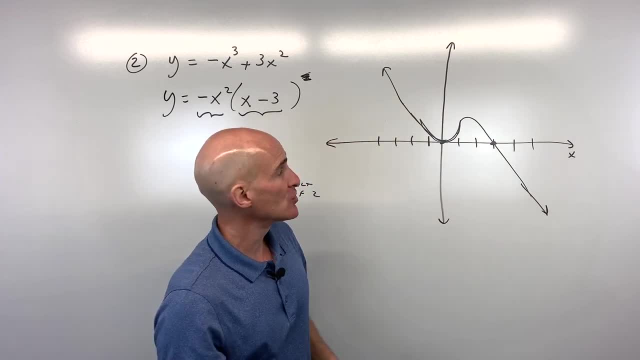 Or how come I didn't just go like that? And again, this is just a rough sketch. You could plot some more points in between. you know these x-intercepts, okay, these zeros, and get an idea. You know that would be good. 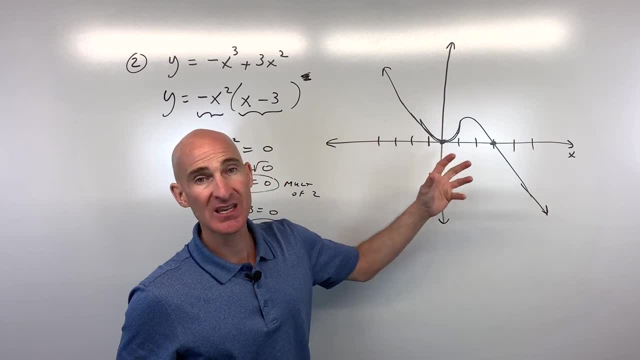 But for this video, for right now, we're just talking about a basic sketch using those three components. Okay, number three, this one's got a little bit of everything in it, so it's a really good example. But before I dive into it, I'm going to talk a little bit about the basic sketch. 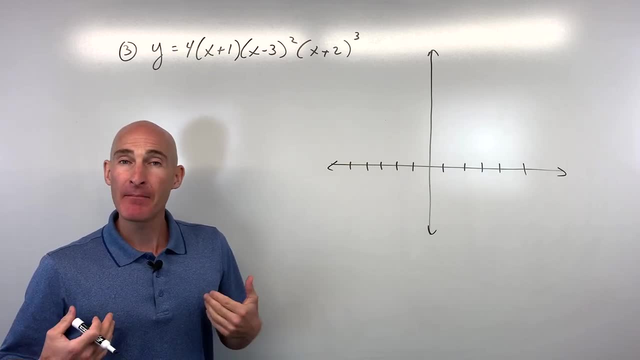 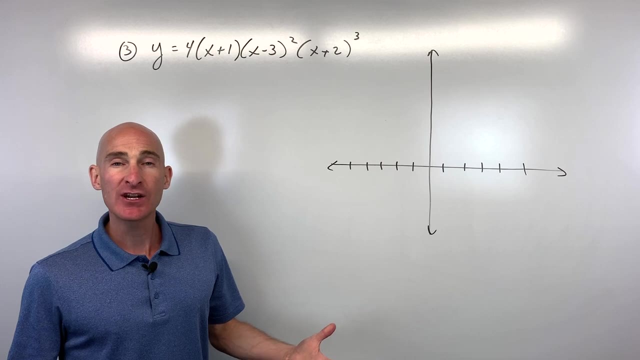 Before I dive into that one, if you're new to the channel and we're meeting for the first time, my name is Mario of Mario's Math Tutoring and I tutor students every day, full-time, And basically what I try to do is take what I learn about, what helps students the easiest, the quickest, the best. 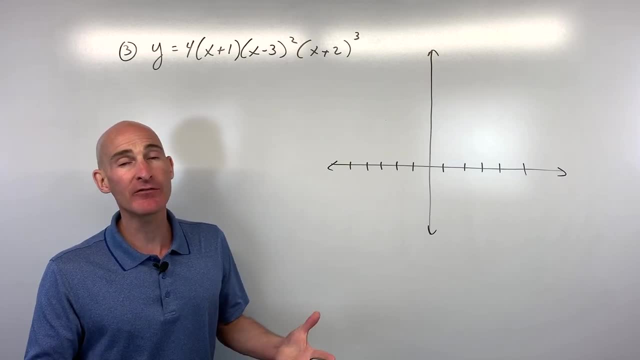 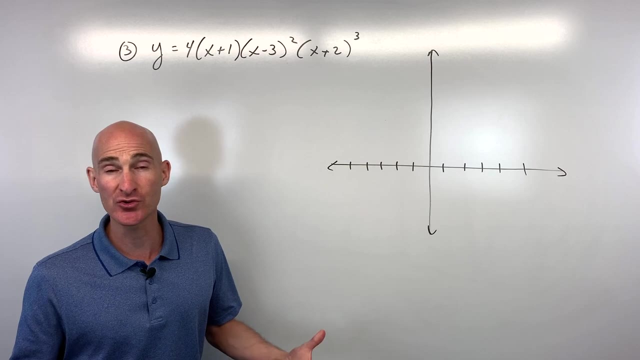 in my tutoring sessions and I bring it to these videos so that you can benefit from my tutoring as well. So the channel's all about making learning math less stressful, so you can raise your grade, pass your class and go on to pursue your dreams. 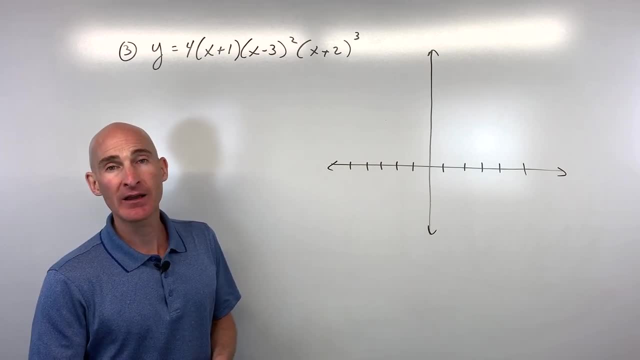 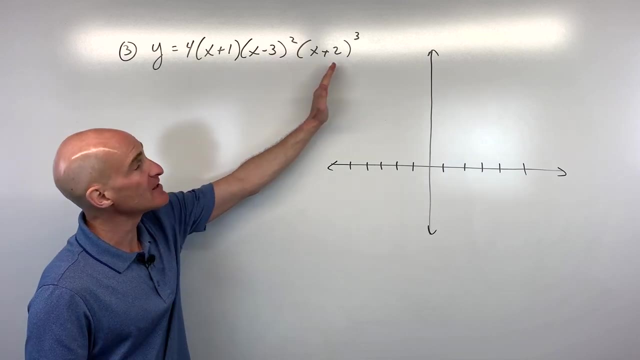 So, if this is something you're interested in, check out more math videos, My YouTube channel, Mario's Math Tutoring, And let's dive into this last example now, The first thing we want to do. this one's all nicely factored for us, right? 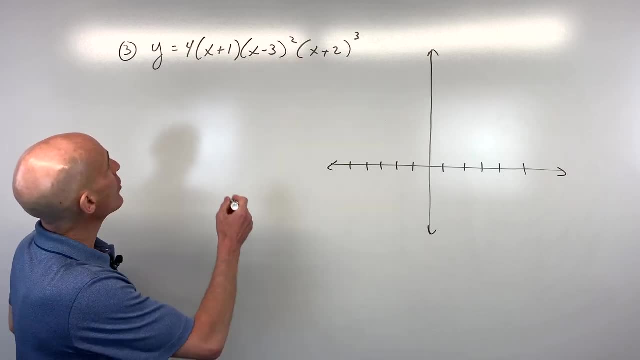 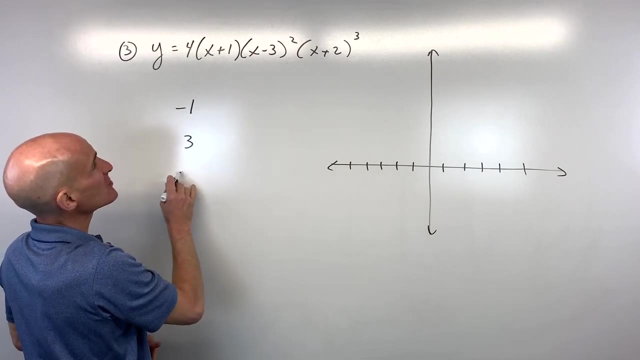 So let's look at the zeros. If we set the factors equal to zero, you can see we're going to get x plus one equals zero, which gives us negative one. x minus three equals zero, which is going to give us three. 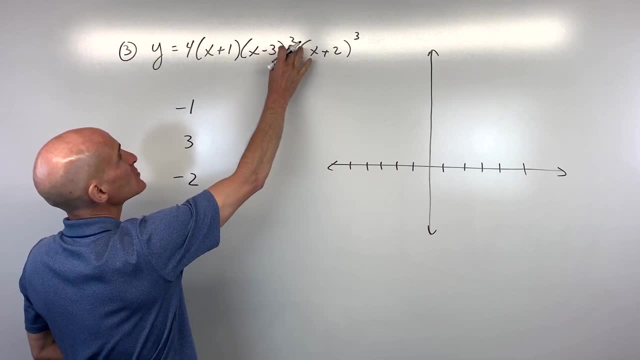 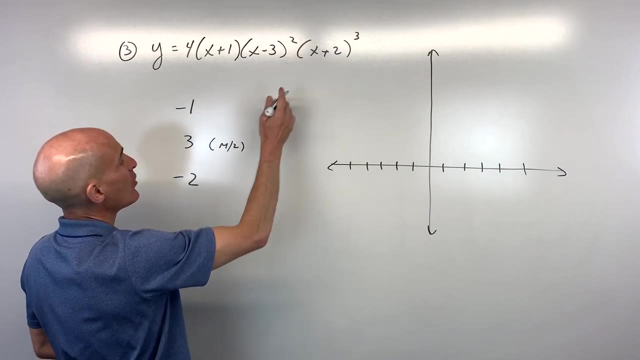 And then here, when we set this one to zero, we're going to get negative two. But notice how this one has a multiplicity of two. So I'm just going to put multiplicity of two, something like that. one has a multiplicity of 3, so I'm just going to say multiplicity 3,, something like that. 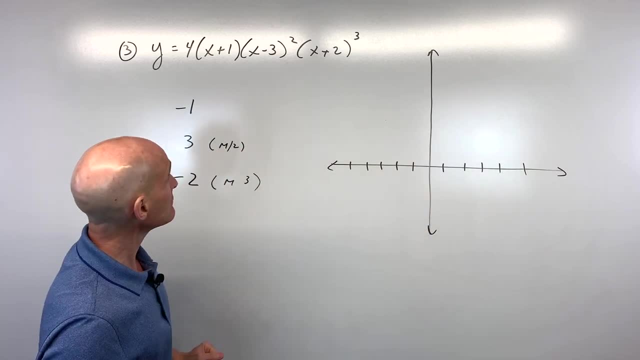 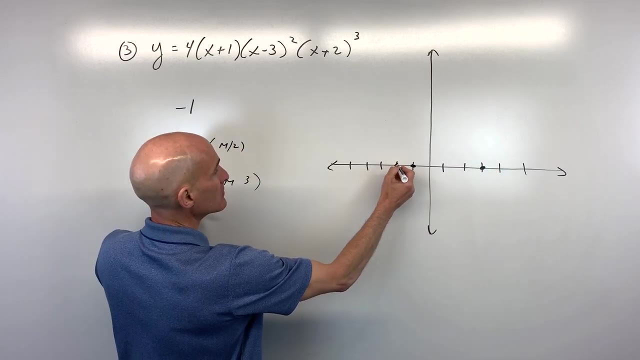 just to kind of remind us when we go to graph it. So here you can see the x-intercepts: negative 1,, positive 3, and negative 2.. Okay now how about n behavior? Is the graph going to go up to the right or down to the right? Leading coefficient is positive, so we know. 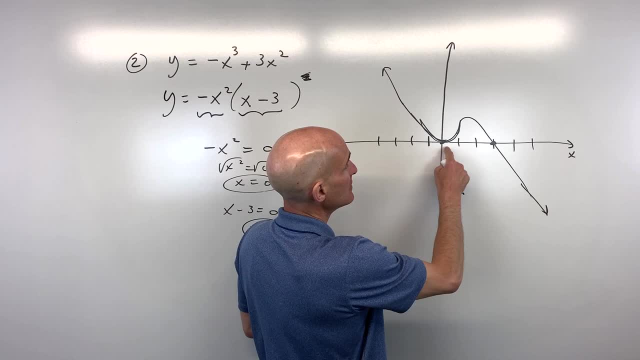 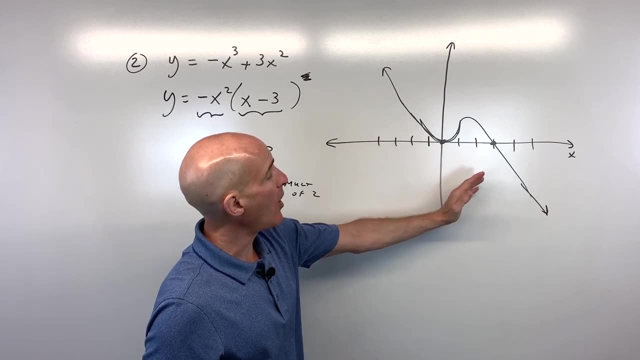 And again, this is just a rough sketch. You could plot some more points in between. you know these x-intercepts. okay, these 0s and get an idea. You know that would be good, But for this video, for right now. 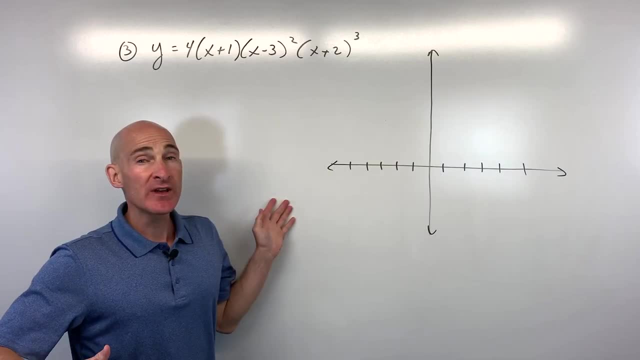 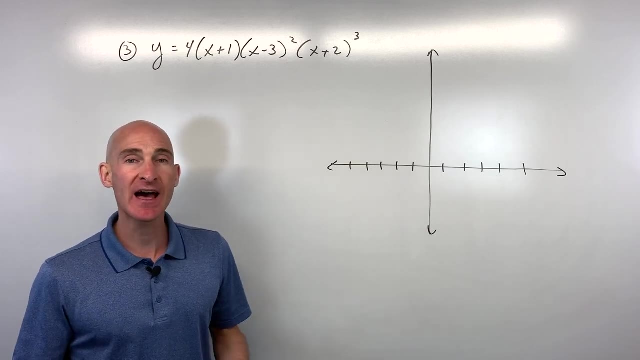 we're just talking about a basic sketch using those three components. Okay, number 3.. This one's got a little bit of everything in it, so it's a really good example. But before I dive into that one, if you're new to the channel and we're meeting for the first time, 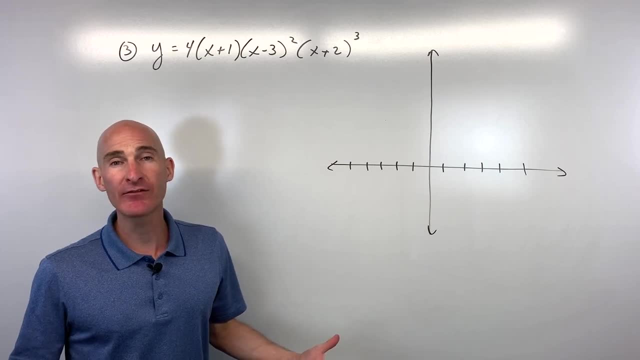 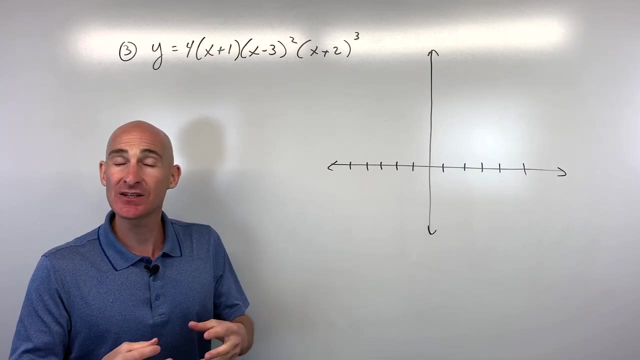 my name is Mario of Mario's Math Tutoring and I tutor students every day full time And basically what I try to do is take what I learn about, what helps students the easiest, the quickest, the best in my tutoring sessions and I bring it to these videos. 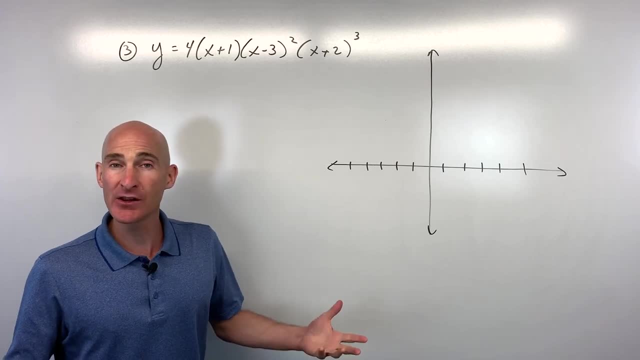 so that you can benefit from my tutoring as well. So the channel's all about making learning math less stressful so you can raise your grade, pass your class, pursue your dreams. So, if this is something you're interested in, check out more math videos on my YouTube channel. 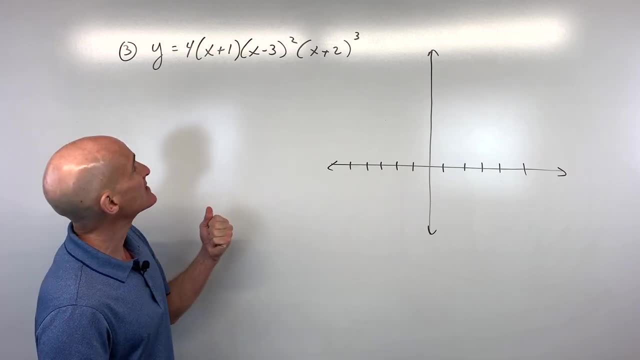 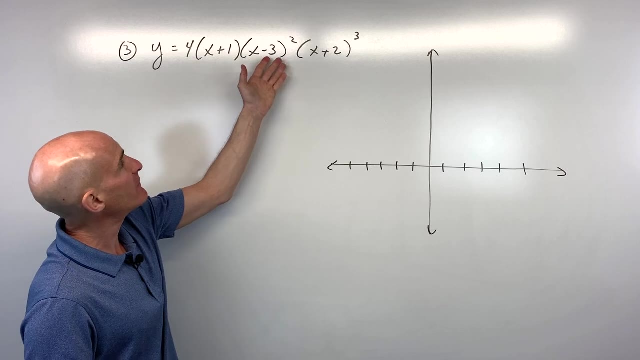 Mario's Math Tutoring. And let's dive into this last example now, The first thing we want to do. this one's all nicely factored for us, right? So let's look at the 0s. If we set the factors equal to 0,, 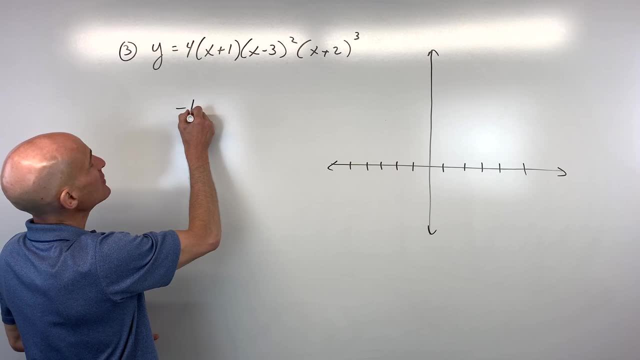 you can see, we're going to get x plus 1 equals 0,, which gives us negative 1.. x minus 3 equals 0,, which is going to give us 3.. And then here, when we set this one to 0,, 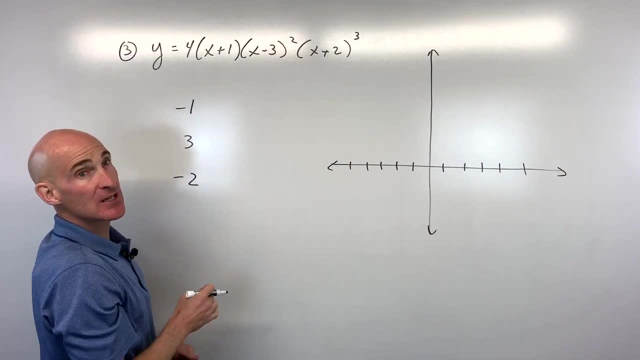 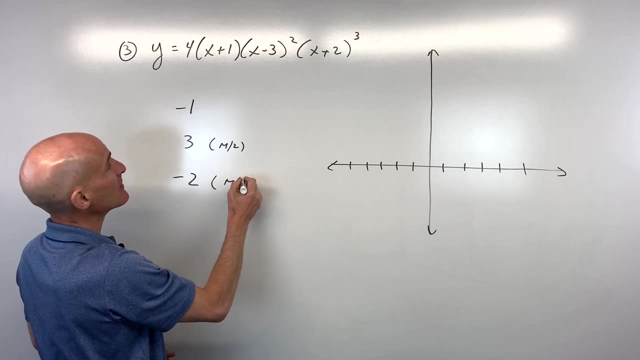 we're going to get negative 2.. But notice how this one has a multiplicity of 2.. So I'm just going to put multiplicity of 2,, something like that. And this one has a multiplicity of 3, so I'm just going to say multiplicity 3,. 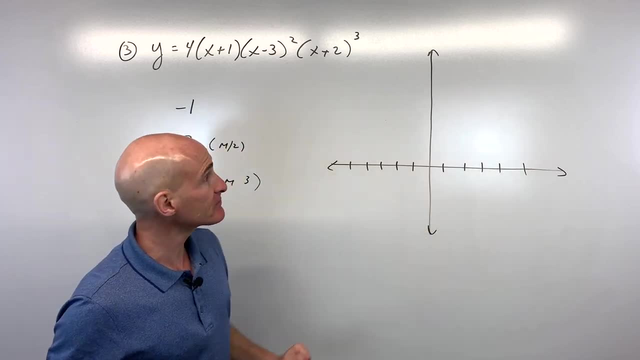 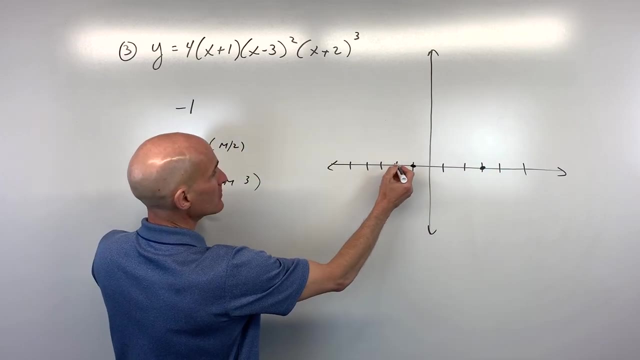 something like that, just to kind of remind us when we go to graph it. So here you can see the x intercepts: negative 1,, positive 3, and negative 2.. Okay now, how about n behavior? Is the graph going to go up to the right or down to the right? 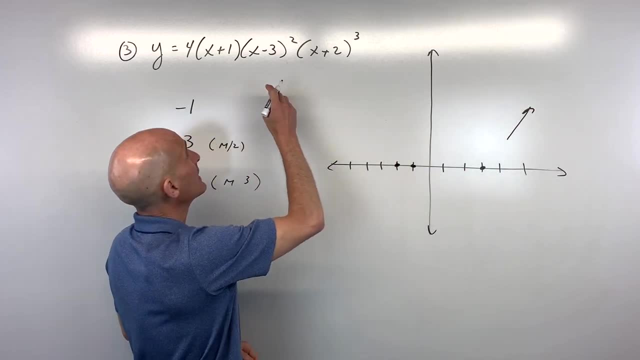 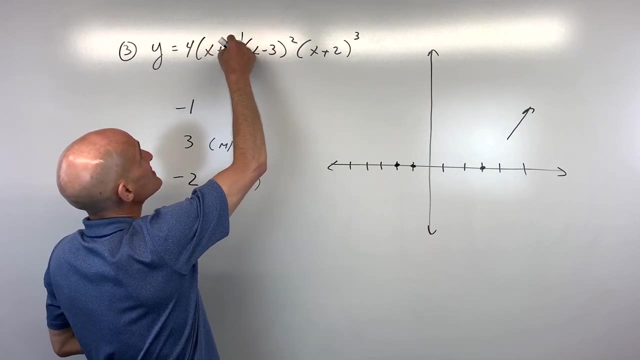 Leading coefficient's positive, so we know that's going to go up to the right. Now what about the degree? You don't want to foil all this out. I mean you could, but it would take you a while. We can just look at these exponents. 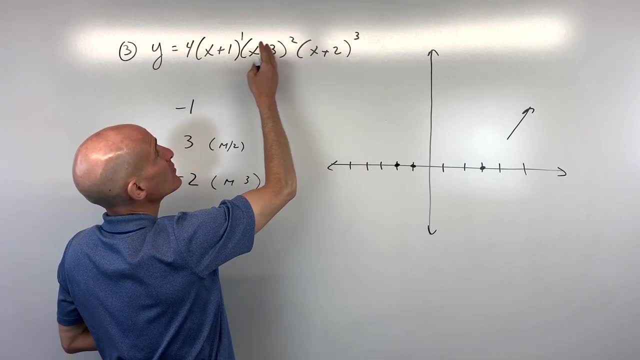 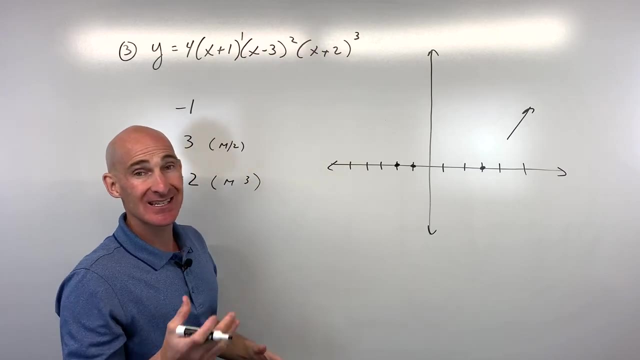 This is x to the first, x to the second, x to the third. When we multiply, what do we do to the exponents? We add them: 3 plus 2 is 5 plus 1 is 6.. So that means that this is a sixth degree. 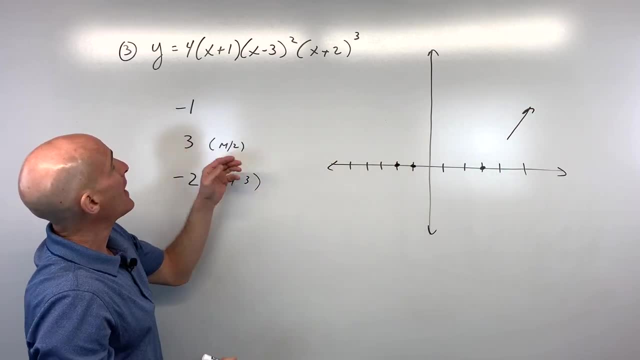 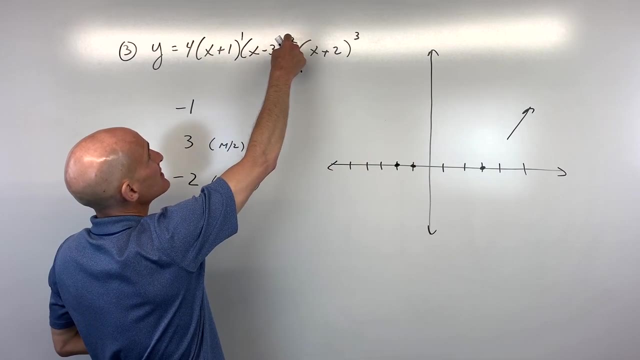 that's going to go up to the right. Now, what about the degree? Now, the degree. you don't want to foil all this out. I mean you could, but it would take you a while. We can just look at these exponents. This is x to the first, x to the second, x to the third. When 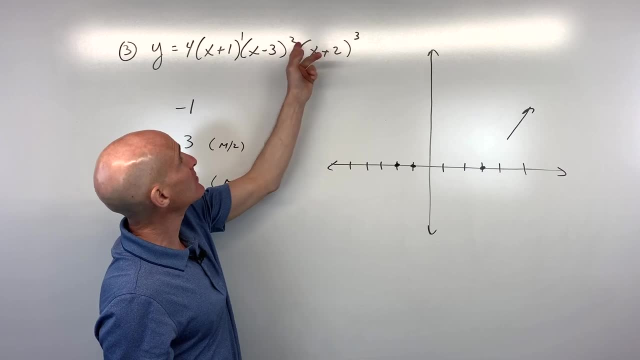 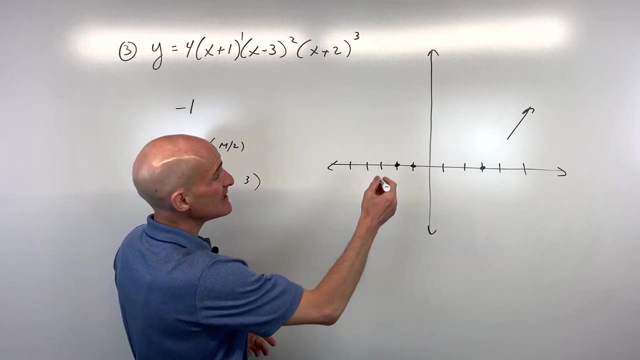 we multiply. what do we do to the exponents? We add them: 3 plus 2 is 5, plus 1 is 6, so that means that this is 6th degree, which is even, and when it's even the n behavior. 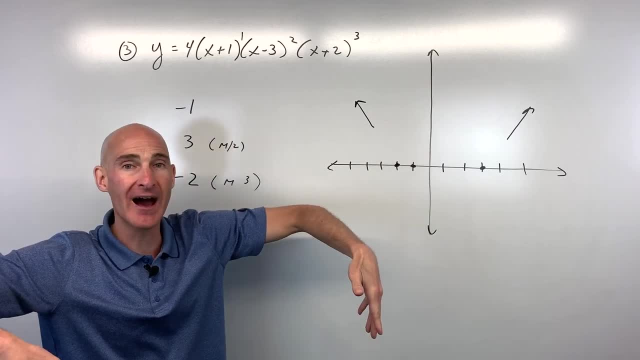 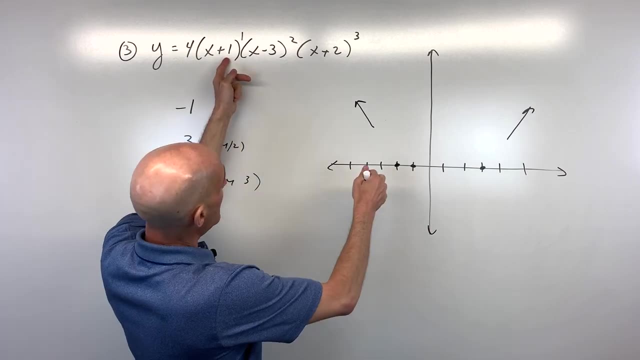 to the right and the left is going to be the same, either both up or both down. okay, if it's odd, opposite. right. Now we get to the fun part: the shape of the graph. So here at negative 2, that has a multiplicity. 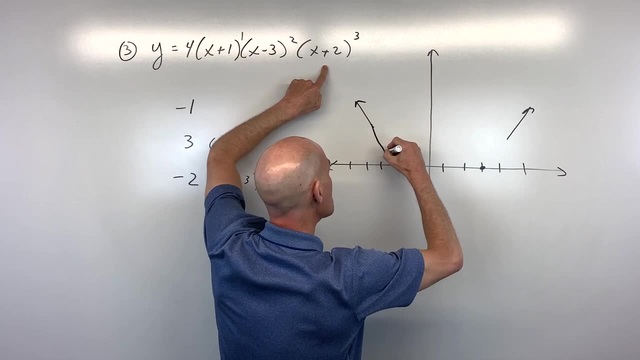 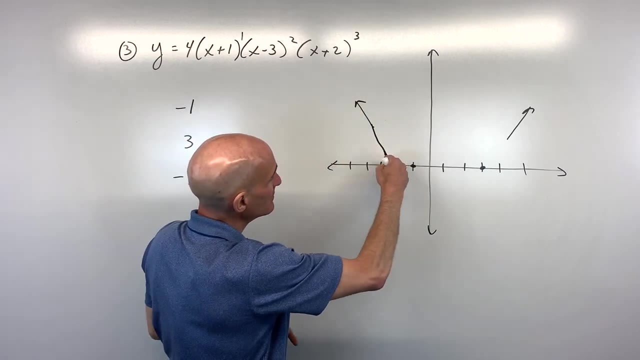 Multiplicity of three. So what that means is, when this graph approaches negative two, it's going to have that cubic shape. okay, If you want, you can draw it straight through, But if you want to be a little bit, give it a little bit better sketch. it's going to. 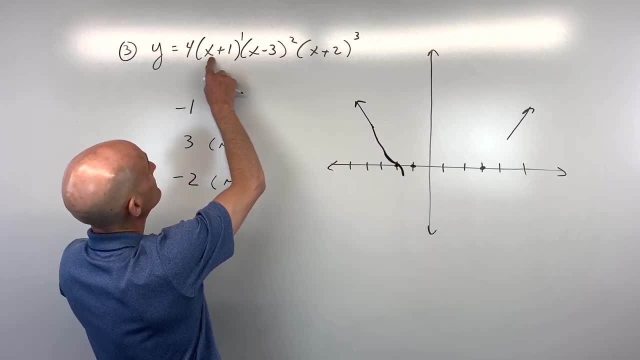 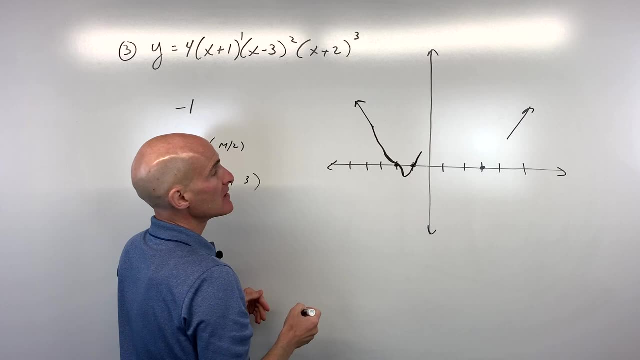 have that y equals x cube shape At negative one. okay, this had a multiplicity of one, which means it's going to go through this point like a line, Kind of just like straight through, like that It's not going to bounce off, It's not going to have that cubic shape. 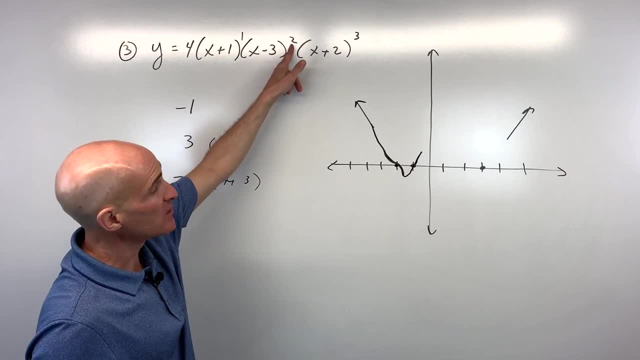 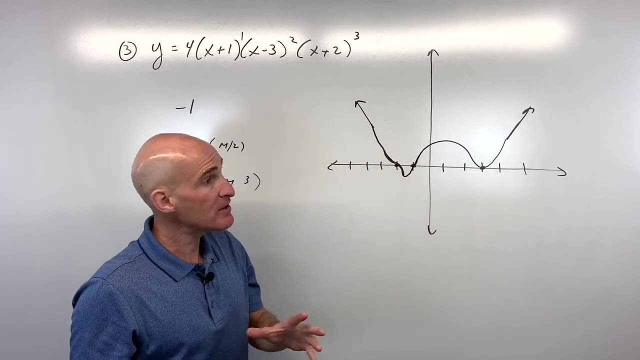 it's going to be like a line, And then the last one at 3, that has a multiplicity of, which means that this is going to have that x squared shape like that parabola shape. at this point, Again, the only thing that's missing are picking some points, maybe in between some of these zeros. 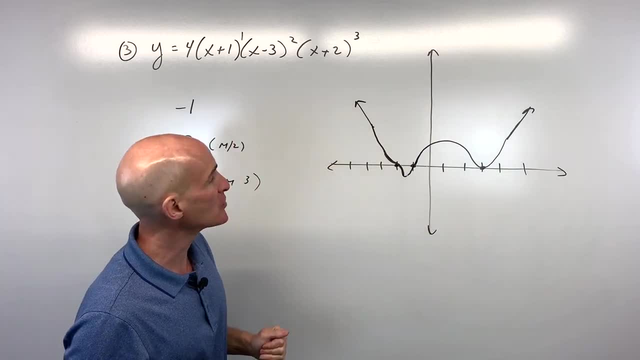 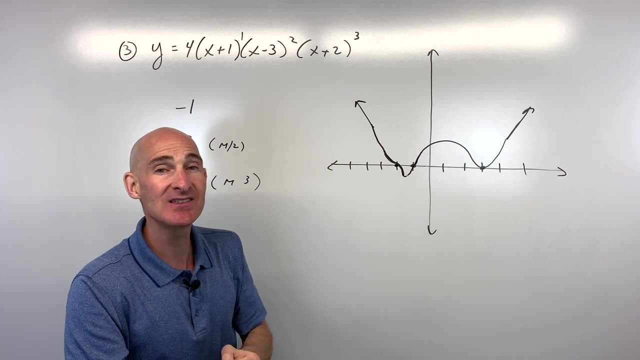 to get an idea about you know how high up it goes or how low it goes, But this is a pretty good sketch of our graph. The things that we didn't cover in this video were Descartes' rule of sines. 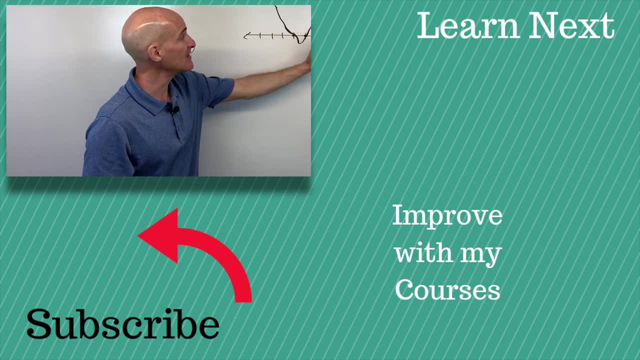 the rational root theorem or rational zero theorem for finding these zeros if you can't easily factor it, And I talk about those things as well as graphing it all together with what we did here in that video right there. So follow me over to that video right there, where we dive into even more depth on graphing polynomials. I'll see you in that lesson. 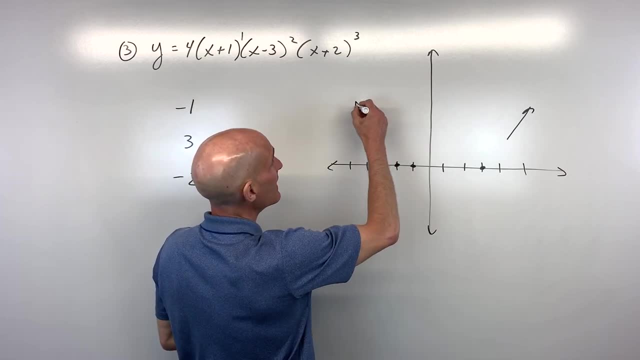 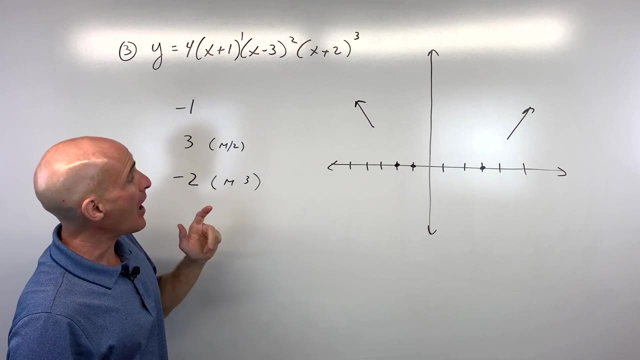 which is even, and when it's even, the n behavior to the right and the left is going to be the same, either both up or both down. Okay, if it's odd opposite. right Now we get to the fun part: the shape of the graph. 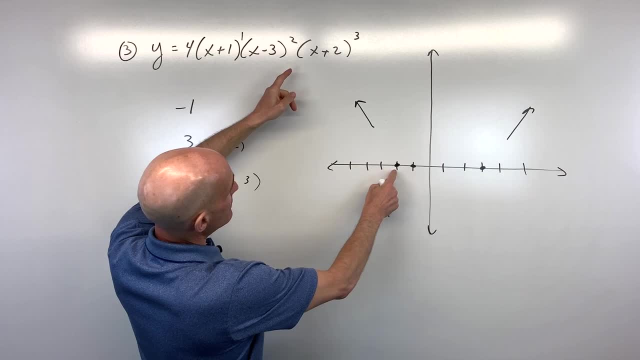 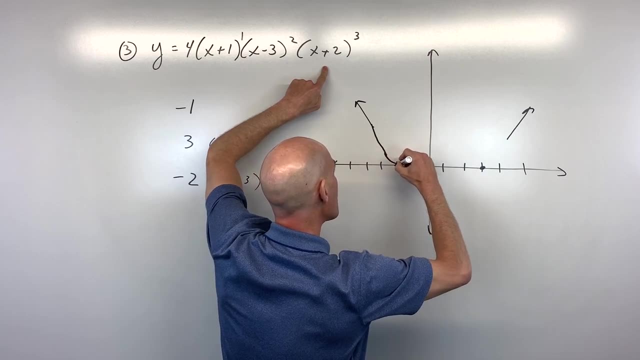 So here at negative 2, that has a multiplicity of 3.. So what that means is, when this graph approaches negative 2, it's going to have that cubic shape. okay, If you want, you can draw it straight through. 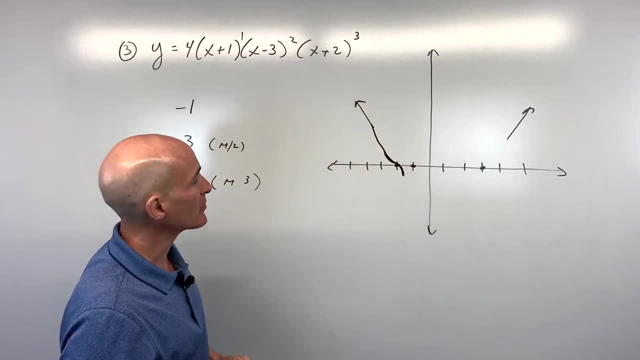 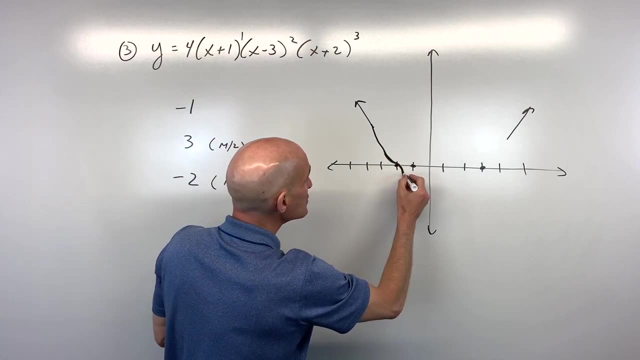 but if you want to be a little bit, give it a little bit better sketch. it's going to have that y equals x, cubed shape At negative 1, okay, this had a multiplicity of 1, which means it's going to go through this point like a line. 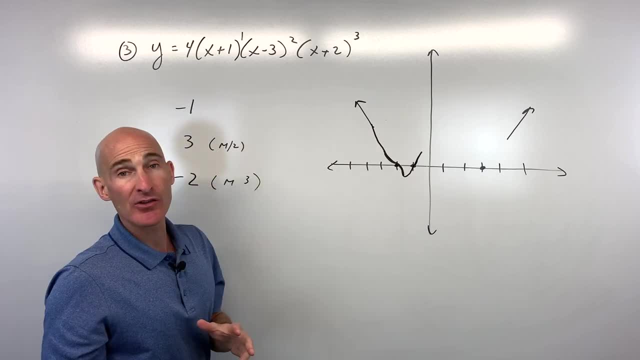 kind of just like straight through, like that It's not going to bounce off, It's not going to move, It's not going to have that cubic shape, It's going to be like a line. And then the last one at 3,. 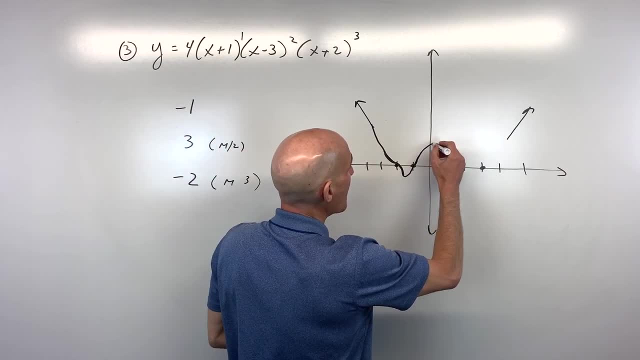 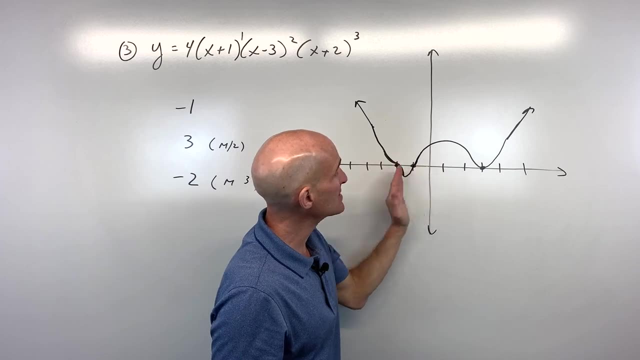 that has a multiplicity of 2, which means that this is going to have that x squared shape, like that parabola shape. at this point, Again, the only thing that's missing are picking some points maybe in between some of these zeros. 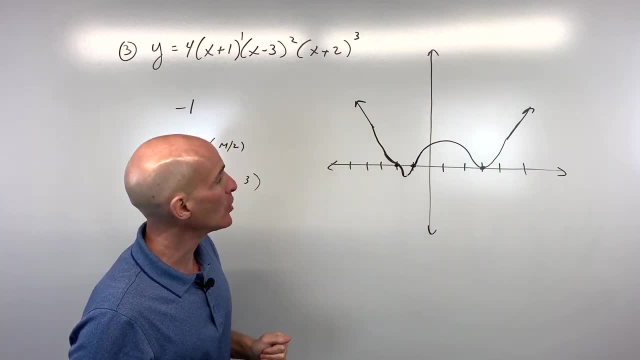 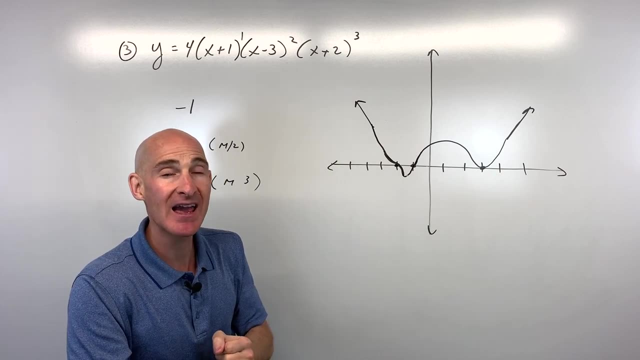 to get an idea about you know how high up it goes or how low it goes, But this is a pretty good sketch of our graph. The things that we didn't cover in this video were Descartes' rule of sines. 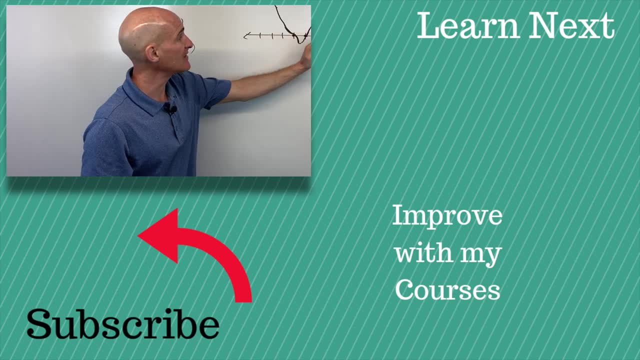 the rational root theorem or rational zero theorem for finding these zeros. if you can't easily factor it- And I talk about those things as well as graphing it all together with what we did here in that video right there. So follow me over to that video right there. 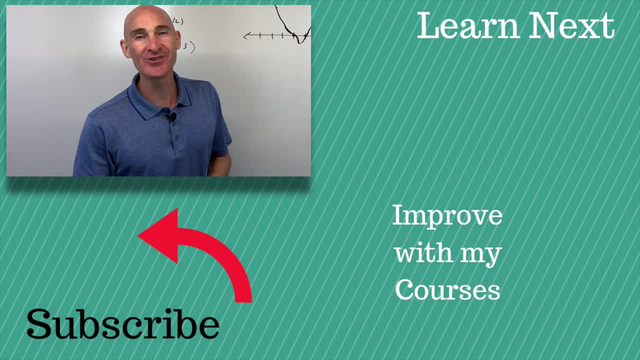 where we dive into even more depth on graphing polynomials. I'll see you in that lesson.